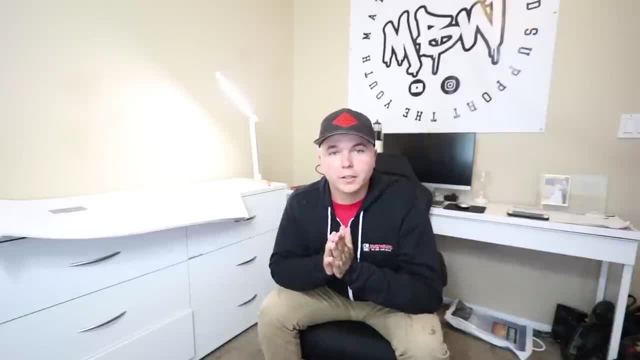 guys know the difference between architectural and structural, go over a couple different things for both. Hopefully, by the end of this video, you took something away from it. Now, before we go any further, I want to show you guys a couple of things that are really helpful. First of all, 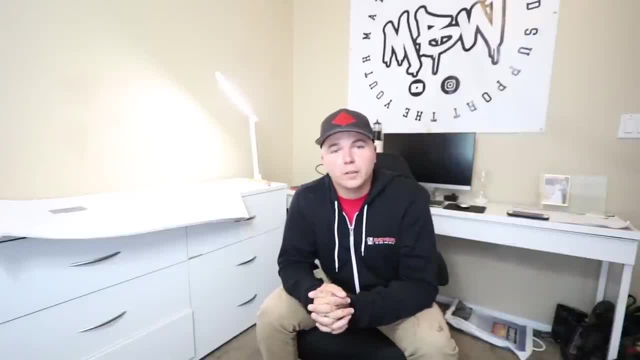 I want to show you guys a couple of things that are really helpful. First of all, I want to show you further. For those of you that don't know me, my name is Matt Piniella. I'm a carpenter from Central California. My father is a general contractor in the area and we have been building 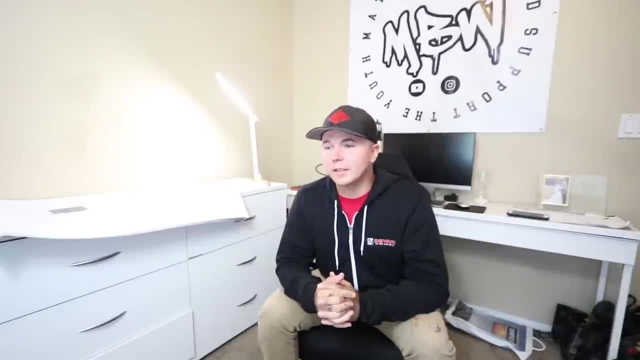 for years now. I dropped out of high school at a young age to start framing and it has become much more than a career for me. I spend my extra time helping you guys out by making instructional content, documenting builds and showing you guys the ways of building If you guys are new here. 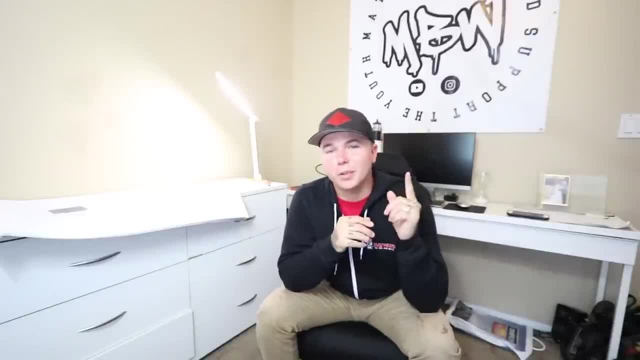 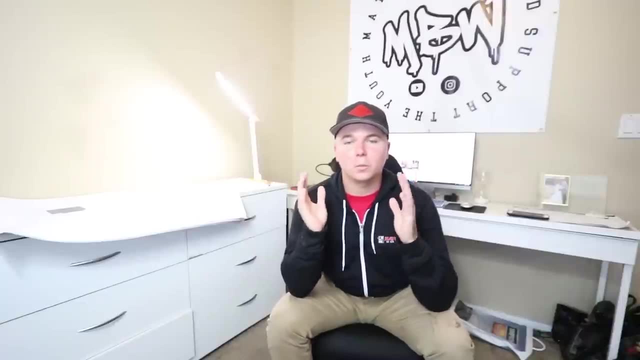 hit that big red subscribe button down below and turn on post notifications. Keep up with everything we got going. This video has absolutely nothing to do with electrical, nothing to do with plumbing concrete, any of that. We're talking framing here. That's all we're going to talk about. 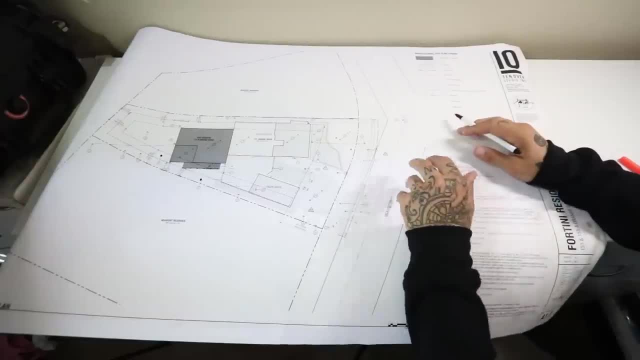 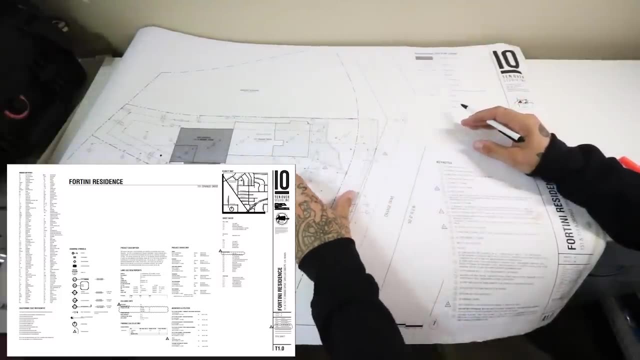 start to finish. Let's dive right in, though. So typically, when you have a set of plans, you have a cover sheet which will have a 3D rendering of the home, along with a bunch of info about where it's located. what's going on, complete scope of work. Since we're only doing 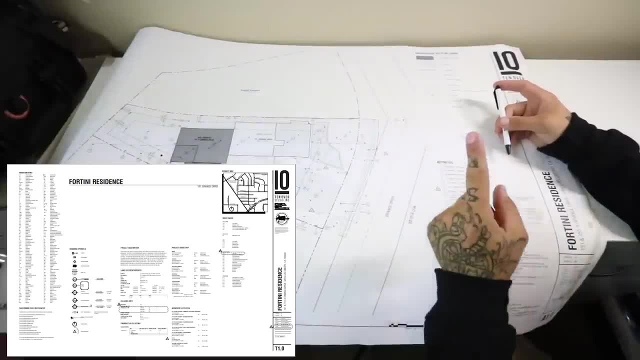 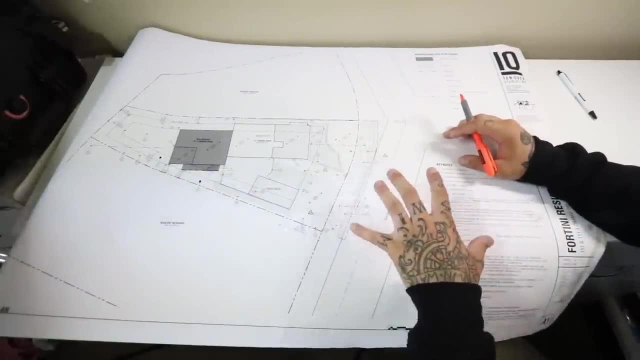 the framing on this project. the only thing we print out is our structural, architectural and elevations. Those three things right there allow us to frame from concrete up. So we are on A1.0.. This is our site. This is going to give us a basic rundown of what's going on on the property. 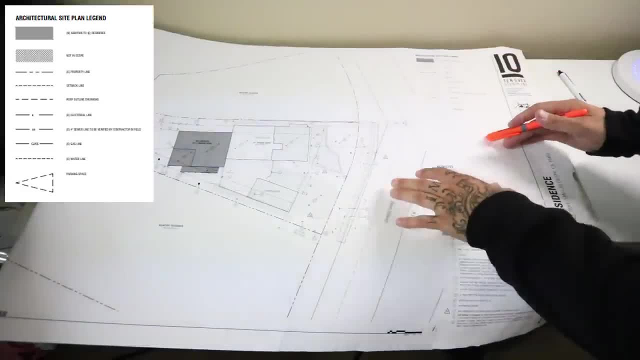 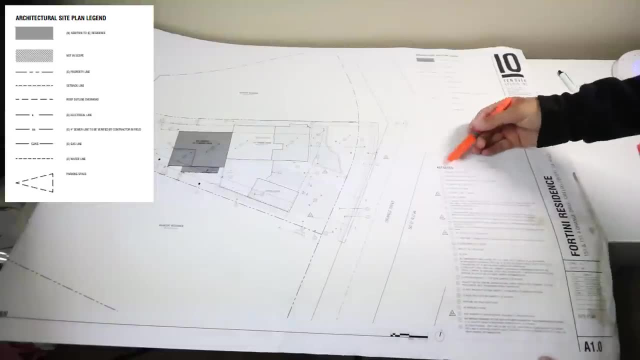 Now think of plans as a puzzle. Everything here has a place. Architectural site plan legend is up here in the corner and it tells you what each individual mark means. You have keynotes here with numbers and circles that go to one spot or another. For instance, number 18 is a new deck. 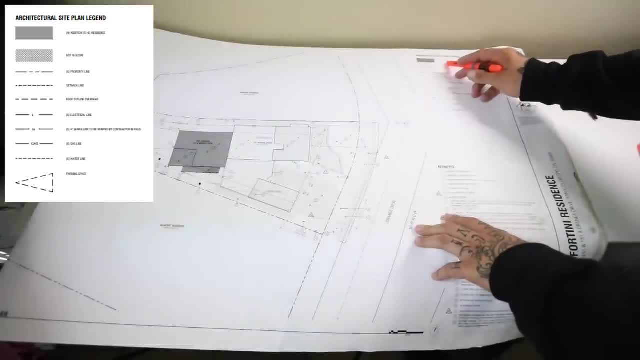 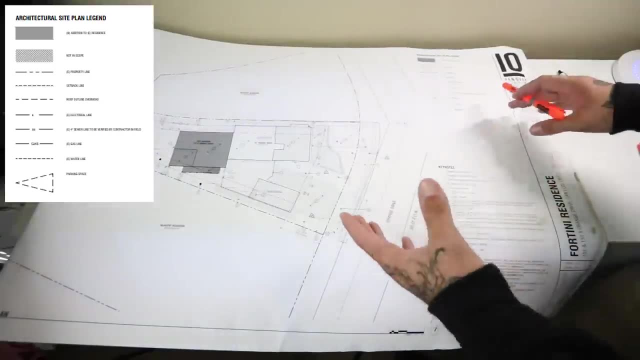 and that's going to be right out there. Up here at the site plan legend you can see new addition to existing residence. That shade right there, obviously it's right out there. It's going to tell you a couple other things. We have E electrical line that runs along the 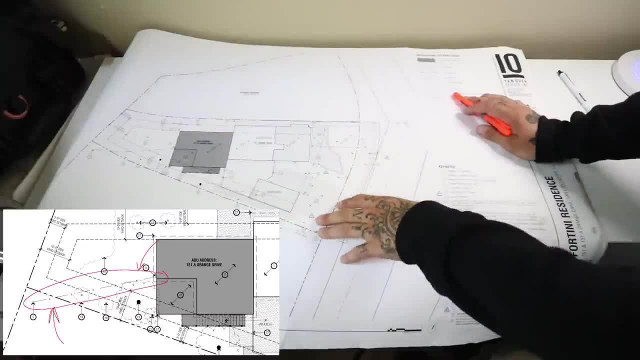 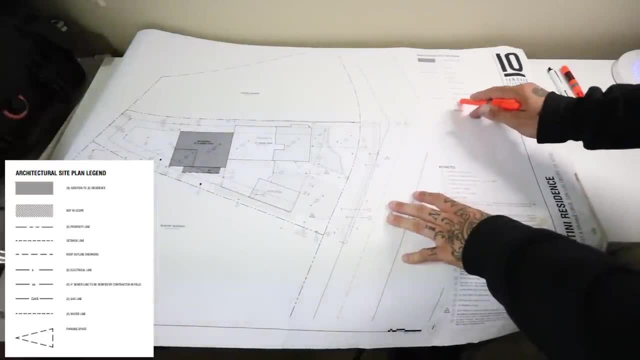 backside there. I'm actually kind of worried about that. It seems like it might be in our way. In the case that it is, we're going to have to have that disconnected. Now, one thing you can check out here: on the site plan you have a water line, a gas line, a sewer line and an electrical line here. 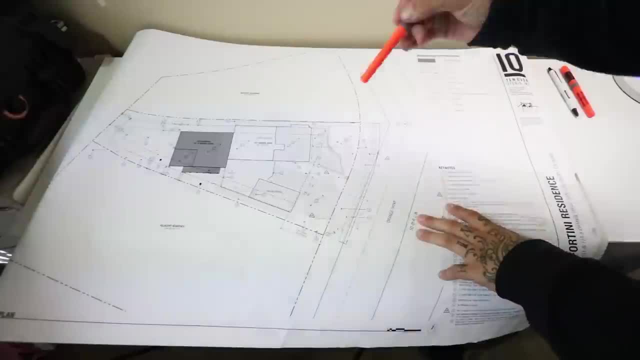 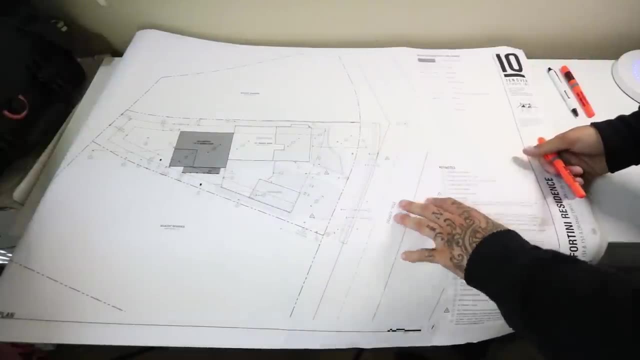 You can find your gas line there, electrical lines right out there, water lines run all over the place. These are things you can look out for before you're either digging or doing other work. Now, since we're framing this project, the only thing we really have to look out for is the 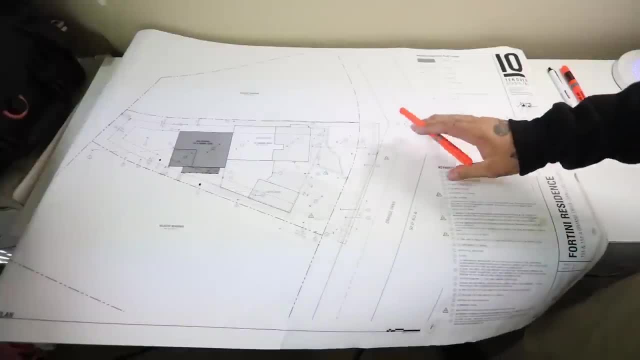 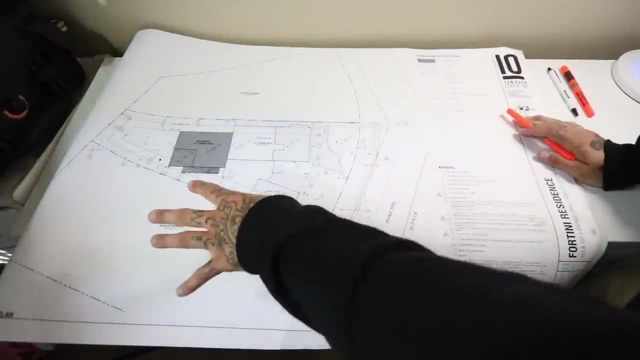 electrical line right there. We don't have equipment on this project since the lot right there is pretty narrow. We actually can't get a lift anywhere on site. We have a home here, home here. street runs along here. Now, another thing the site plan does is tells you exactly. 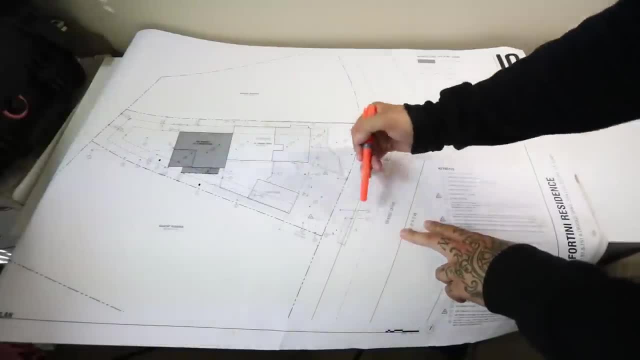 where the lot is and how big it is. As you can see, we've got a little pie shape going on here. There's nowhere to get equipment in. We have an existing garage here, existing home is here, addition goes here and there is nowhere to get a lift anywhere on site. 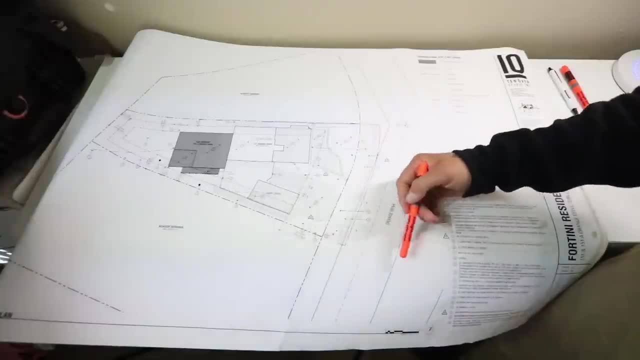 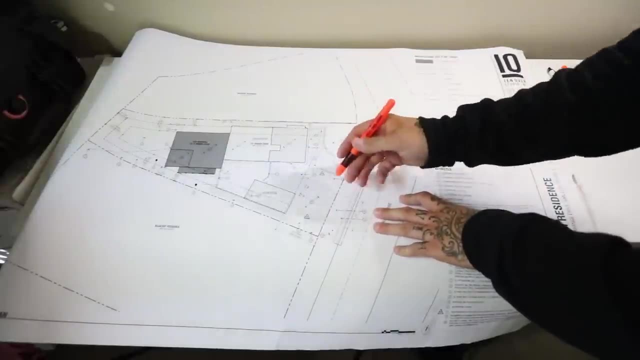 Now our game plan here we're going to have all of our material dropped right here in the driveway. Our laborers are going to pack it back to the addition. That goes for all of our plate, all of our studs, our floor system, roof system, everything These guys are going to put in work. 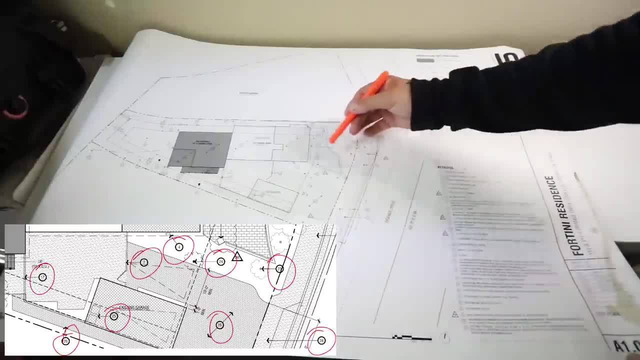 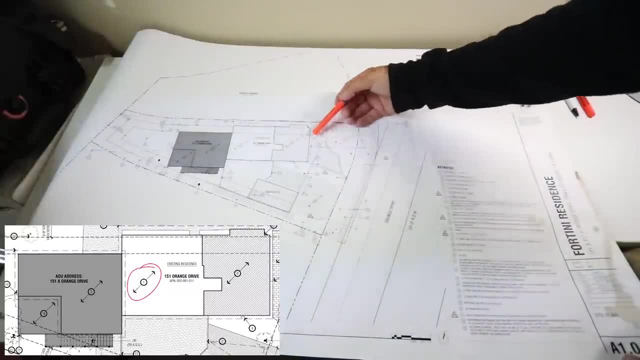 Now on your site plan. here as well, you'll find little circles with numbers inside of them to reference on your keynotes here. Number one, for instance, which is right in here: residents to be renovated. Number two: residents to remain not in scope. So nothing has changed. 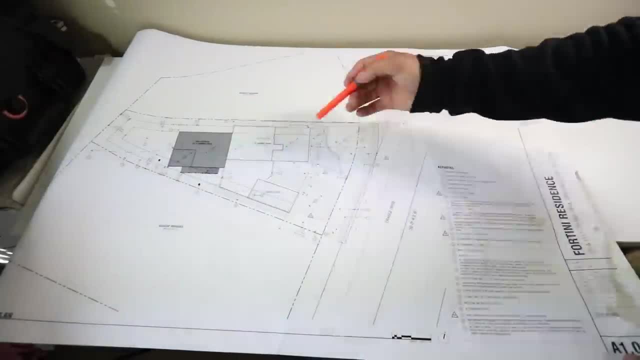 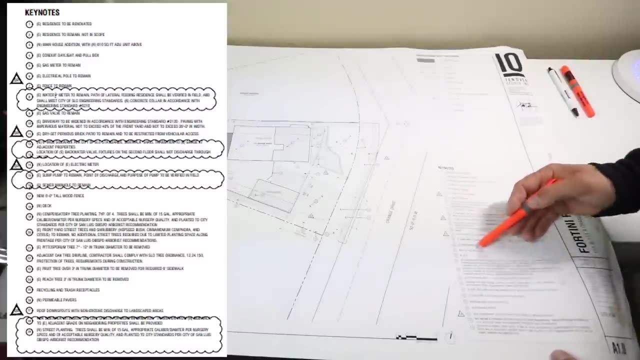 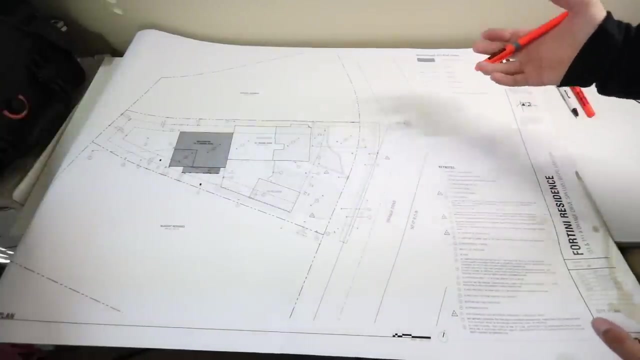 with this side of the home, but this side here is affected. Number three: main house addition with new 610 square foot ADU unit above. Now this here is going to have a list of things for not only the framers but every trade. Now, with the site plan here, they're basically giving you guys a. 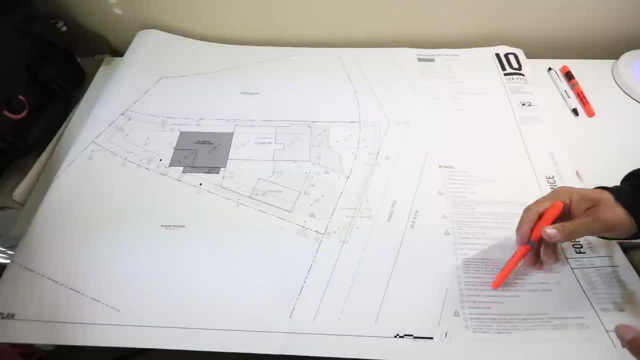 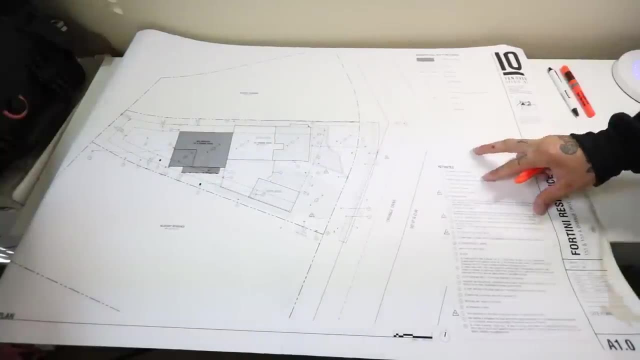 rundown on what's going on. All these keynotes here that you can reference have anything to do from the fruit trees that are being removed to put in the new sidewalk to what's going on with the addition. Now we're going to go ahead and flip pages here and start looking at the 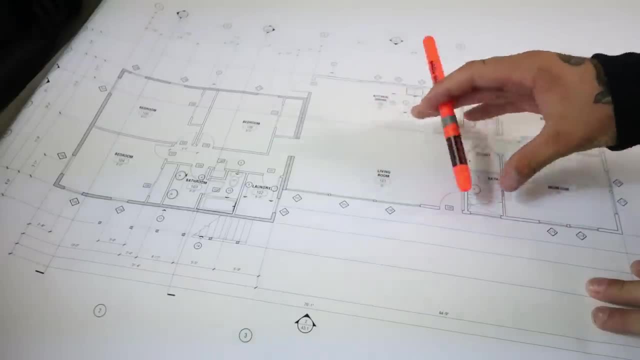 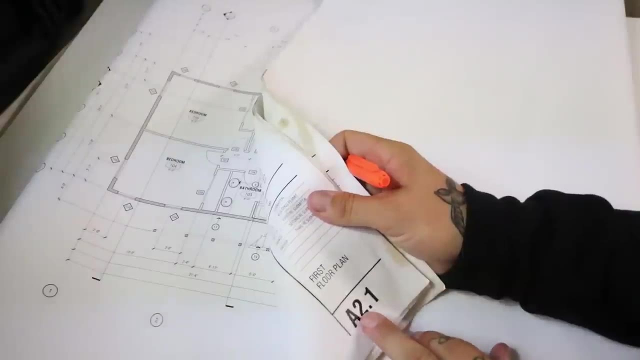 stuff that actually has to do with framing. Now, we're not going to look at any of this here. The only thing we want to look at today is our floor plan that we're going to be building. So we are now on architectural 2.1.. 2.0 was actually a demolition floor plan. 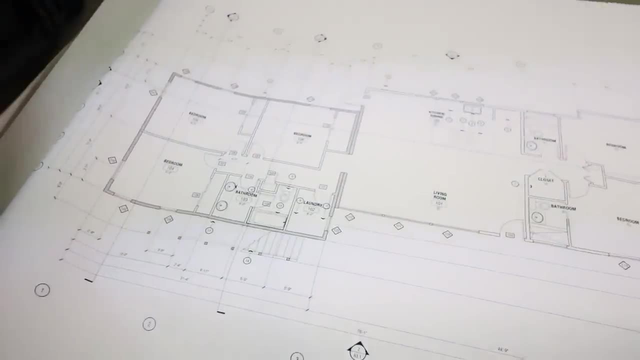 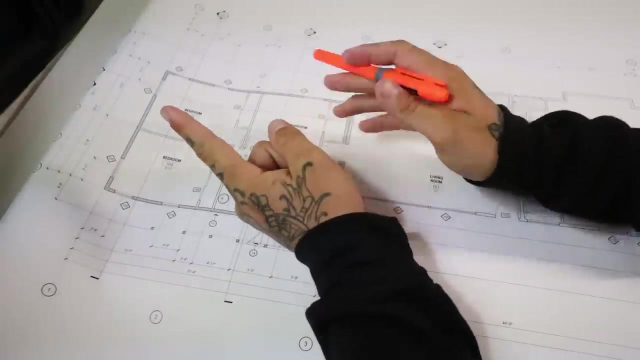 We don't need that because we're not doing demo. One thing to keep in mind when you first start reading plans- that helped me out tremendously- is understanding the difference between an architect and a structural engineer. Architects make things pretty and engineers make things work. Here we have the floor plan. 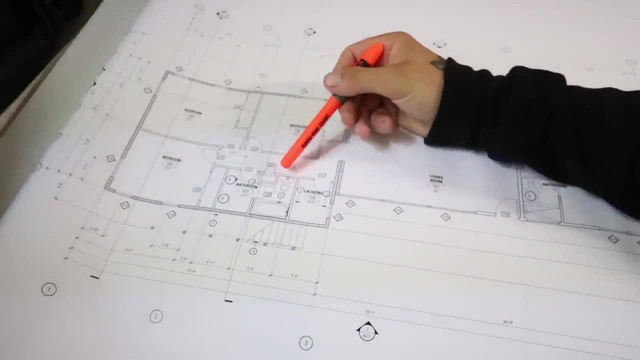 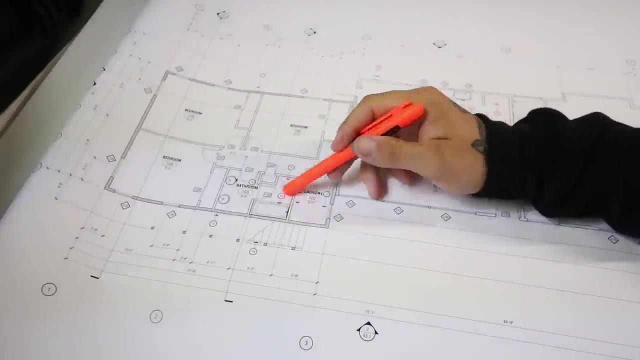 for the addition that we're going to be framing. Architects draw in things like the toilet here, the bathtub here, two sinks and a hallway closet. Engineers are not going to give you any of that info and not going to show anything. They're simply going to show what they want to make: the building up to code. 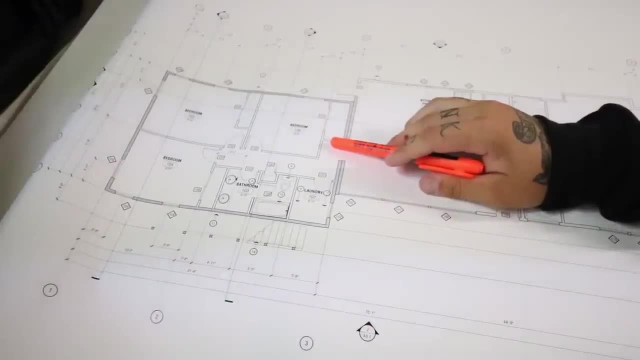 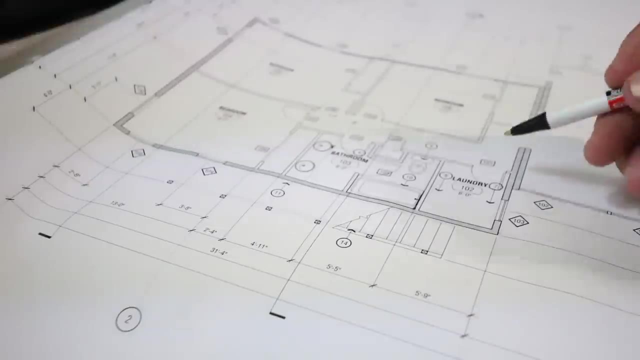 While the architect here is going to explain exactly where all these windows are going to go. Now, the first thing we're going to do when we get on site here is snap this wall along here Five and a half over. snap another line there. That's going to be for that wall. 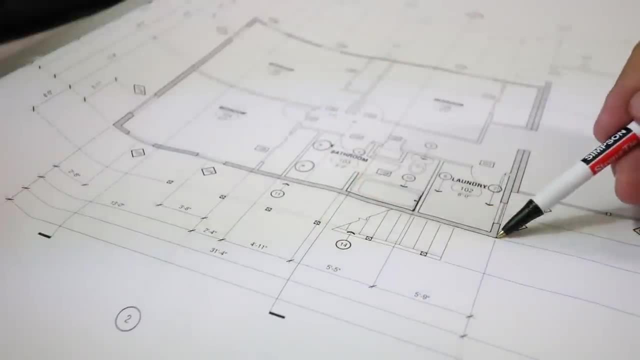 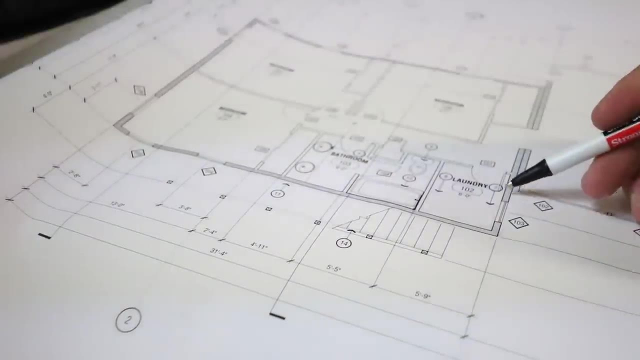 Now from there, you can see here 31 foot four Hooking building over to there. Now what that's going to do, by pulling 31 foot four from corner to corner on both sides, is going to make sure that we are perfectly parallel. We don't suggest following concrete, because concrete isn't always perfect. 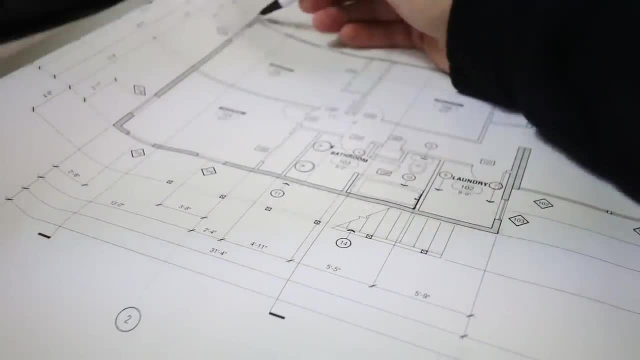 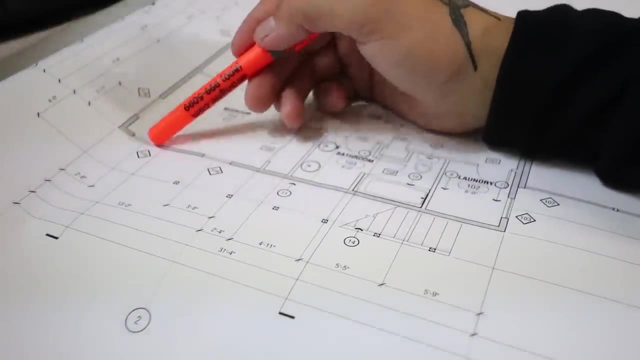 In the case that this is 31 foot four and this may be 31 foot five, you're out an inch already. You don't want to build like that. So now, before you lay out studs in this wall, you should make note of where your windows are and lay those out first. 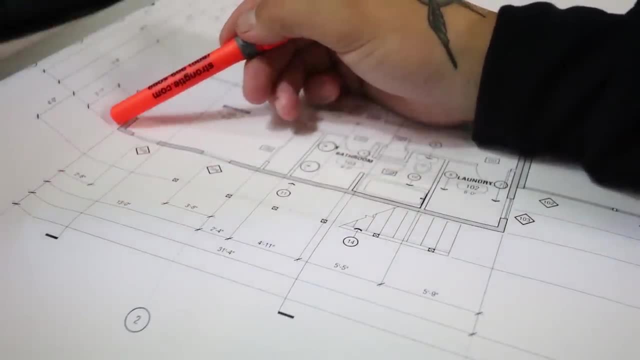 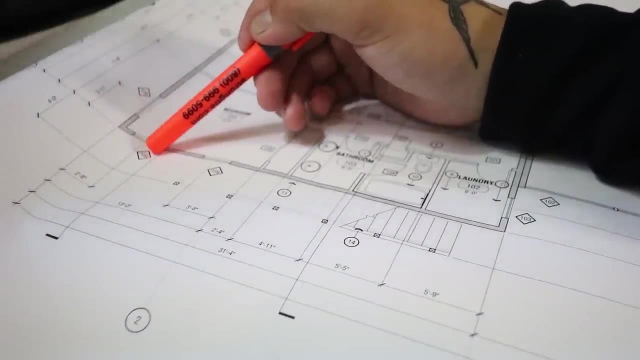 Now, as you can see, here we have two foot eight hooking outside of plate to center of the wall, So we're going to lay out studs in the middle of that window. Now you have 105 written there and a little diamond That is going to be used for reference on your window and door schedule. 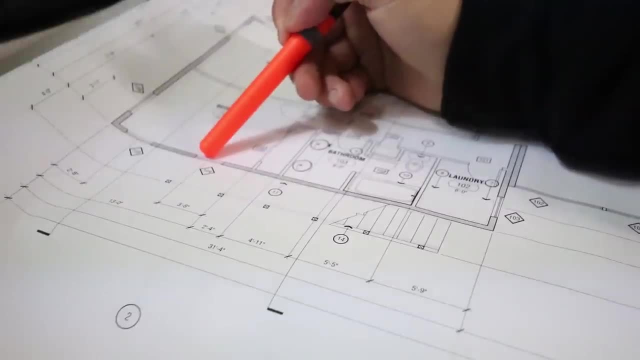 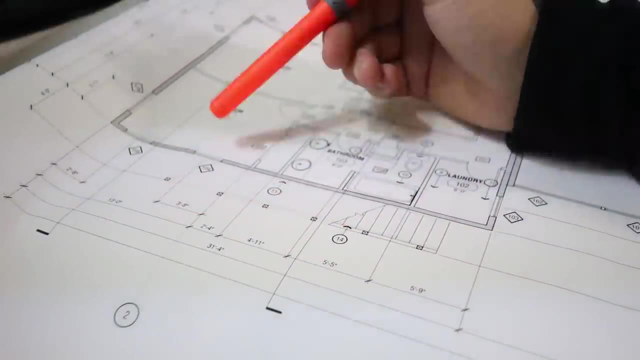 which we'll get to in just a second. So now that you've laid out that window there, we're going to lay out the one right next to it. Typically they would have another number in between and you would just mark center, But this one, as you can see, we've got one, two, three, four, five numbers to your center. 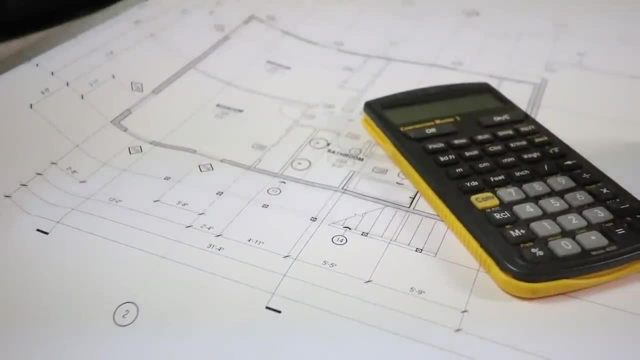 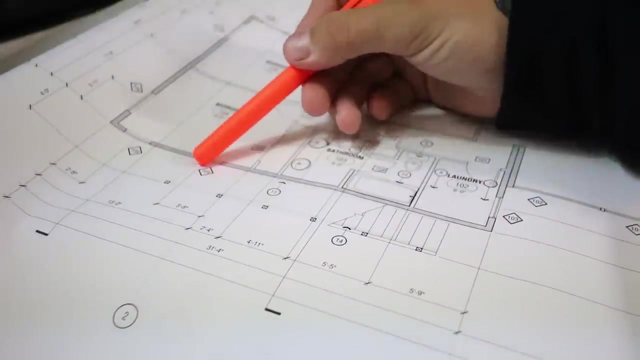 This is where our construction calculator comes in handy. We have five foot nine, Two foot four and three foot eight, 22 foot one, So 22 foot one, hooking outside to center of your window. From there you could find out what size 104 is and pull accordingly and lay out that window. 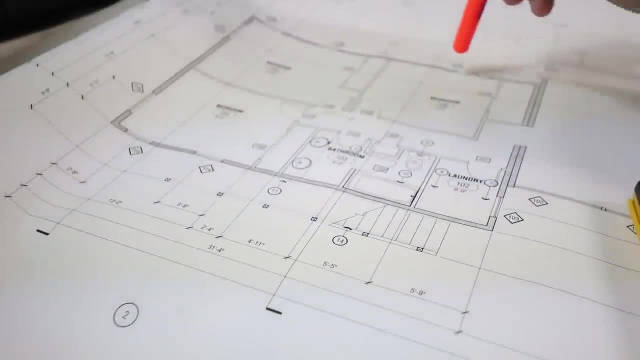 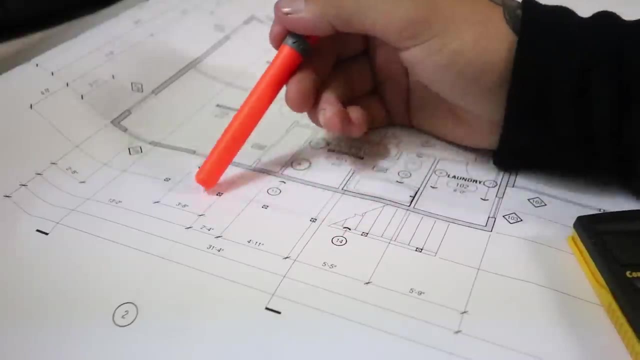 Now it's going to be the same exact thing all the way around. whether it be a door or a window, they all lay out the same. So you have these marks here that determine where your center is going to be, And these are all things listed on the architectural. 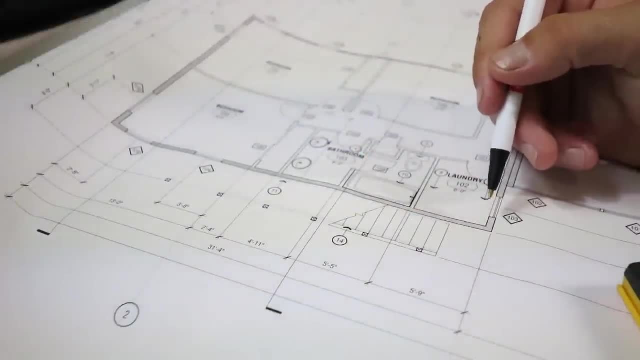 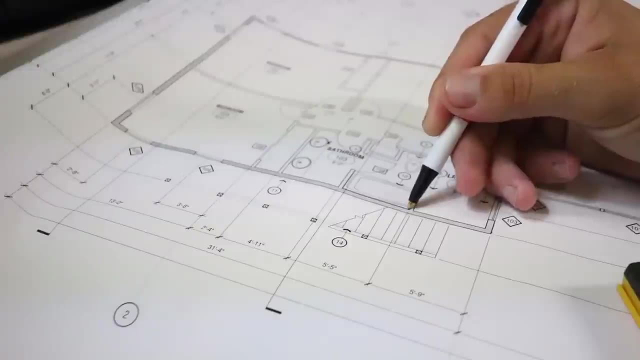 Now, before any of your plating goes down, you're going to snap lines on your slab which you guys will see in our build series starting tomorrow. You would hook that corner there and go five foot nine. You give yourself a mark and go back three and a half. 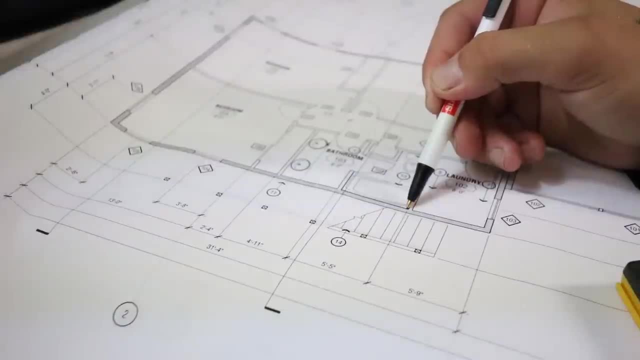 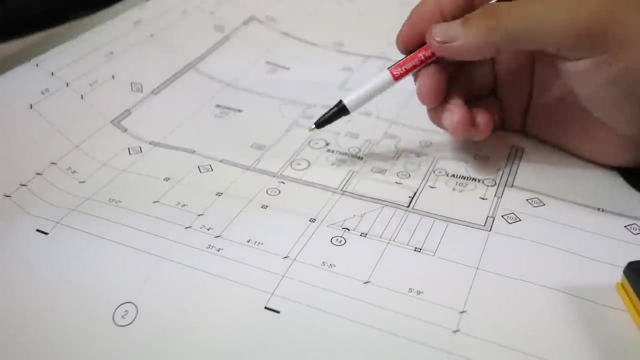 And that is for that interior two by four wall. So now you would butt that wall right there and pull five foot five over the next one, Go back three and a half to there And that's that wall From there. you keep doing that until you have all of your walls laid out. 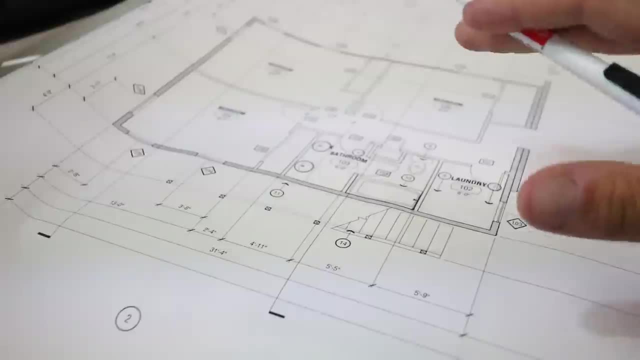 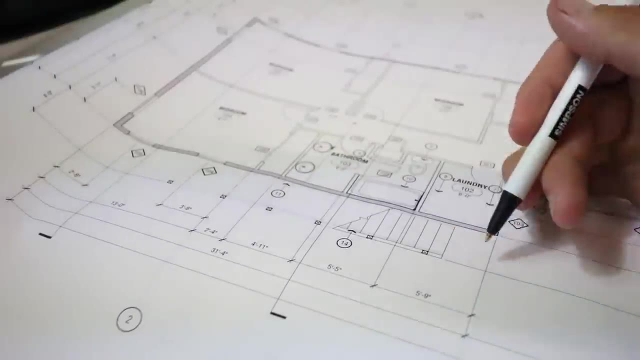 And that is how we will do it for each and every wall in this home. So what I'm going to do for you guys is actually wear a GoPro head mounted for this whole entire build, And you guys will be able to follow along as we build this house. 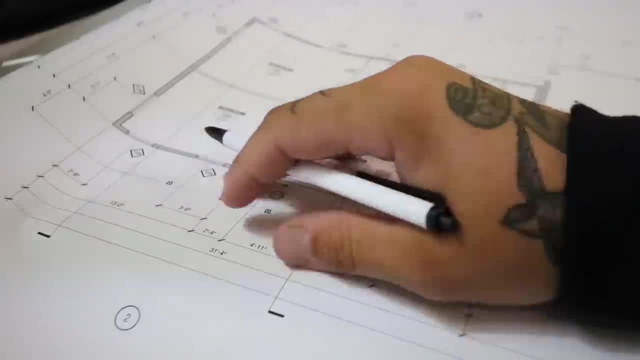 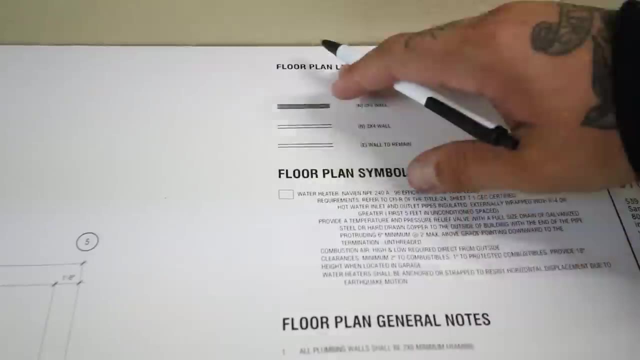 And you can reference the plans, what we're talking about right now- to what we're building on this edition. Not only will you guys get to see it here on paper, but you'll actually get to see it on video as well. So now, on every page, you're going to have something that looks like this: 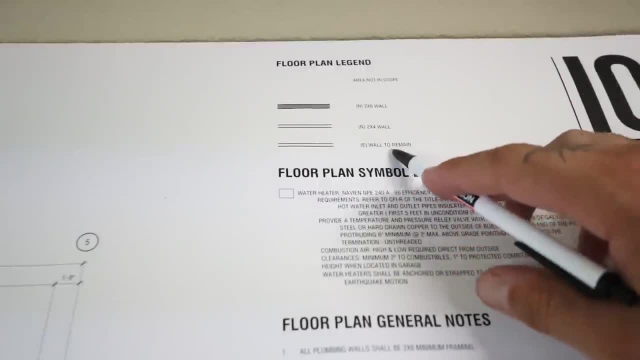 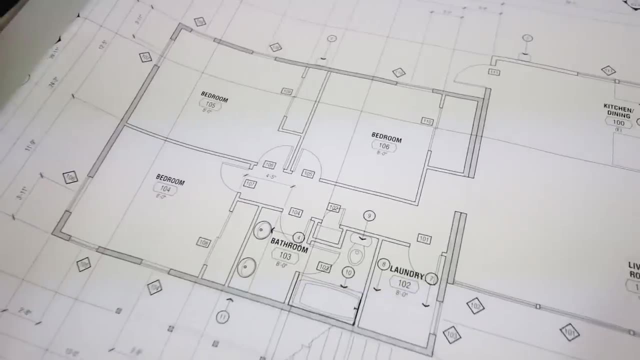 And this is going to tell you exactly what each of these walls mean. You're going to have a existing wall to remain, a new two by four wall, new two by six wall and an area not in the scope. So now, as we come back over to here, you can see that this is going to be a new two by six wall. 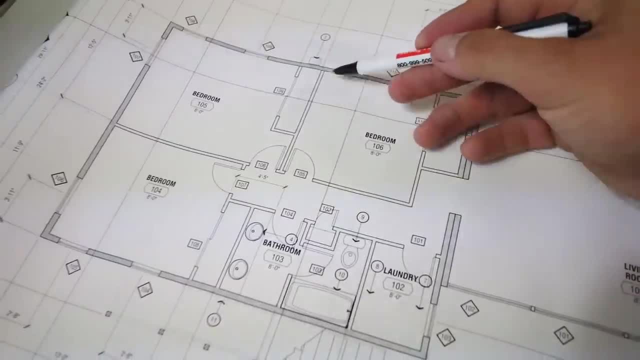 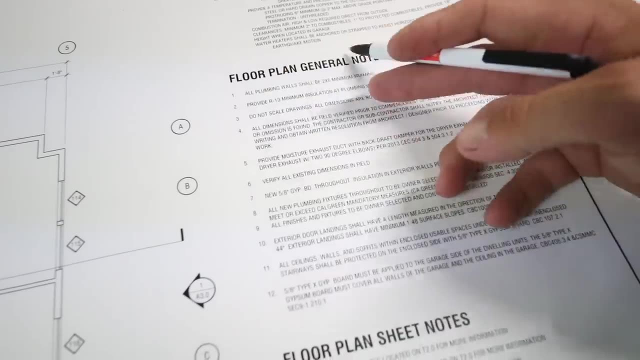 here new two by six wall all the way along the outside Interior. two by four wall is new. And then over here, all of these walls are nothing but white lines because all of this is existing. We have a floor plan general notes section as well, which will tell you different things. 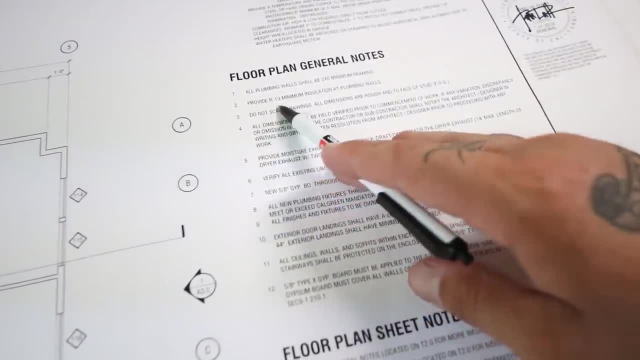 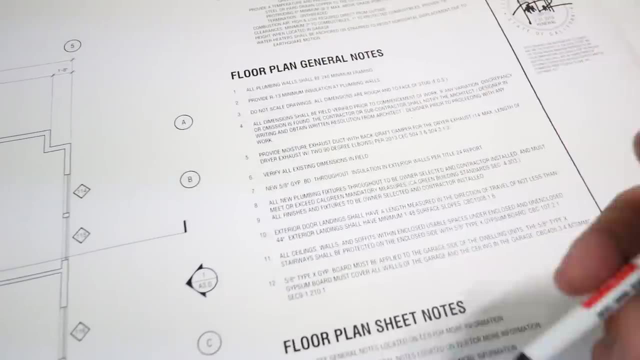 such as: all plumbing walls should be two by six minimum framing. provide R13 minimum insulation at plumbing walls. All of this is info that may be needed As far as our framing goes. there's only a couple of things we're actually going to take away from this. 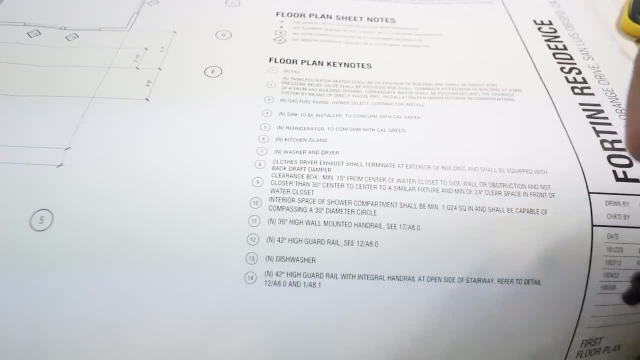 Now, like I explained to you guys, architectural tells you exactly where everything's going to be placed, as far as the toilet goes, the sinks, showers, kitchen island, washer and dryer, so on and so forth. None of this has to do with framing, so we're going to go ahead and skip through this. 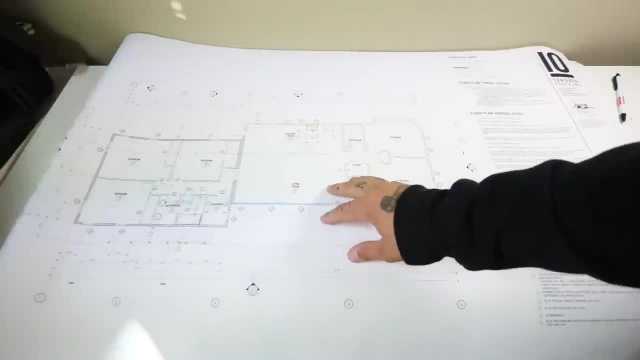 If you guys have any interest, you guys can pause it and read it. Now, when we get to structural, you're going to notice that none of these numbers are on there. You have to go off the architectural floor plan to figure out where all of your other 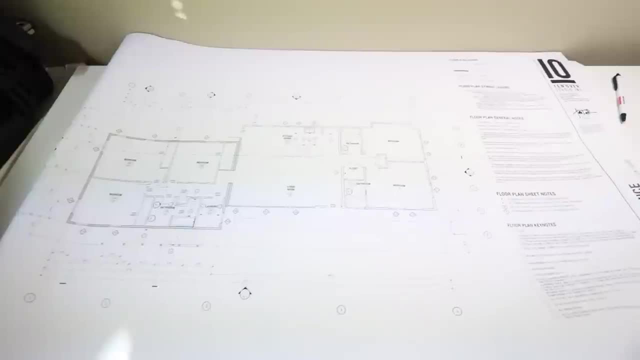 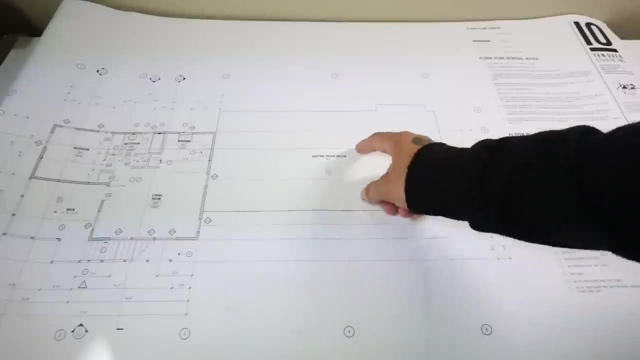 walls are going to be along with where your window and door openings are. We're going to go ahead and flip pages. Now we're on A2.2, the accessory dwelling unit floor plan. Now, this is the upstairs floor plan here. 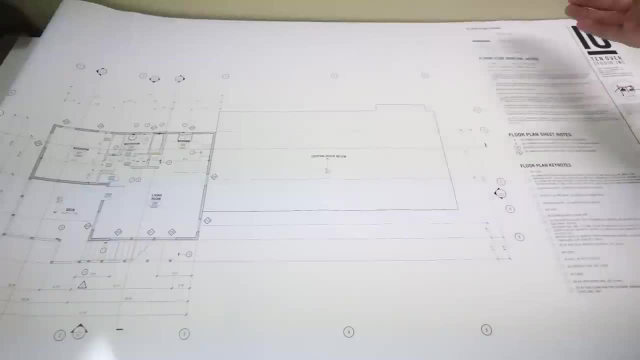 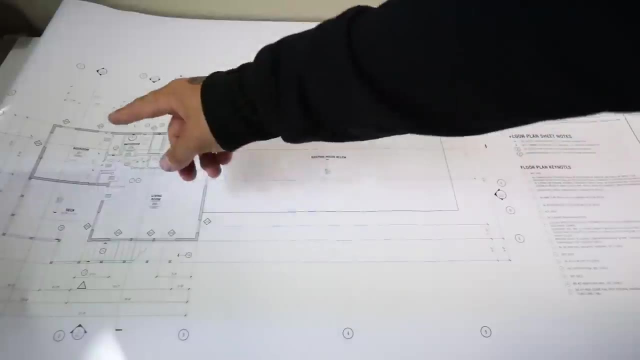 The same exact thing goes here. We have the floor plan, legend, general notes, plan sheet notes and our plan keynotes. We're not going to be looking at these, We're going to check out this right here Now. as you can see, it's the same thing as down below. 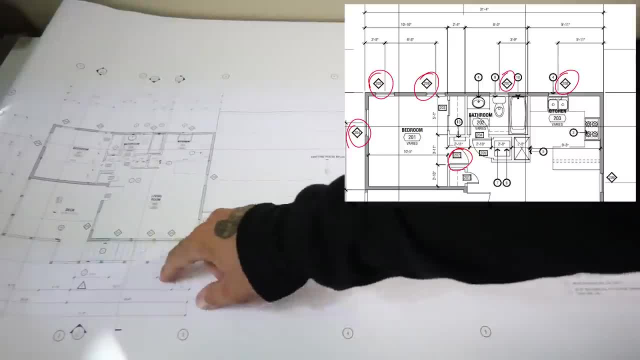 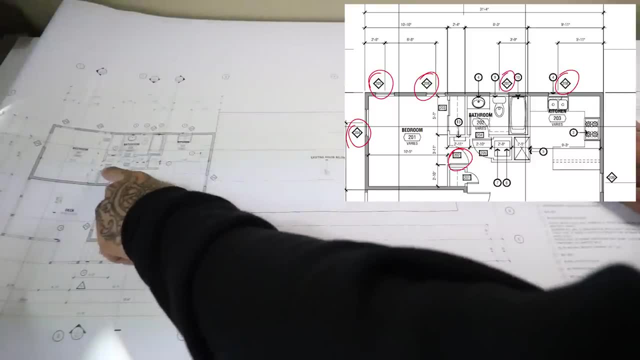 We've got more windows in here, center marks laid out on each one of them, center marks laid out back here as well. All of these diamonds are for our window and door schedule. We have all of our windows. We have our door. 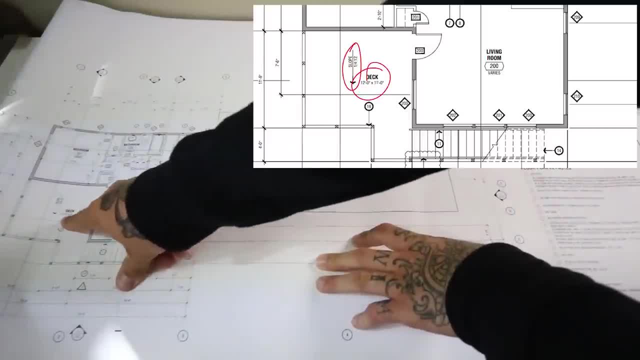 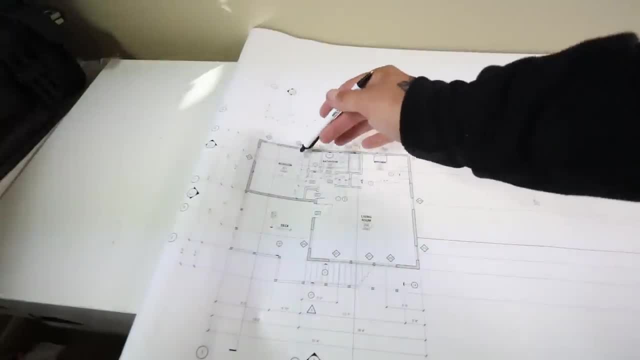 It's number 202.. Now this out here tells you that we have a deck 12 foot by 11 foot quarter per foot slope sloping that way. Now, since we covered layout and how we lay out our windows, our doors and all of our 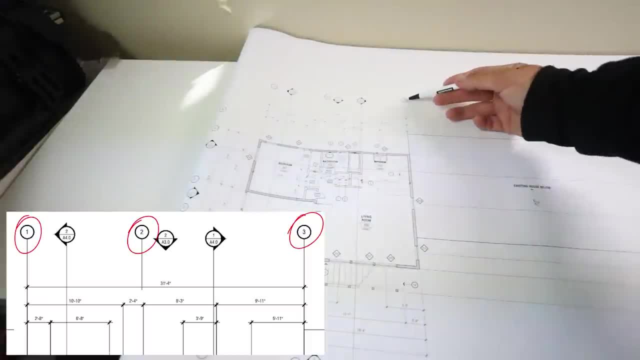 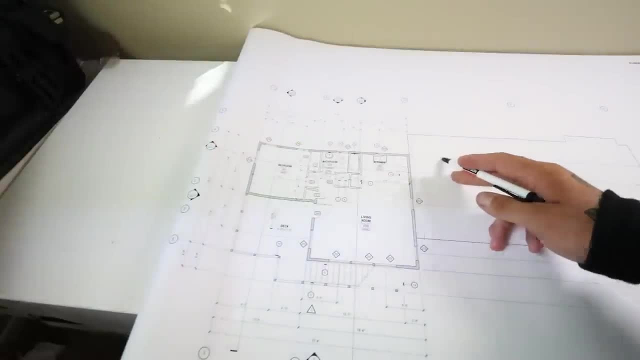 plates down below. we're going to talk about something else. You can see the three here: two one A, B, C. These are called grid lines. We have B runs all the way through, Three runs all the way through here. 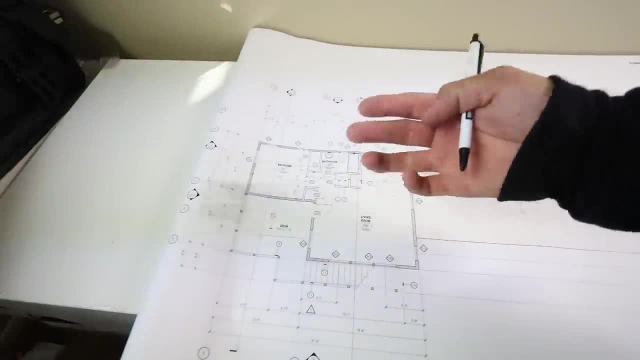 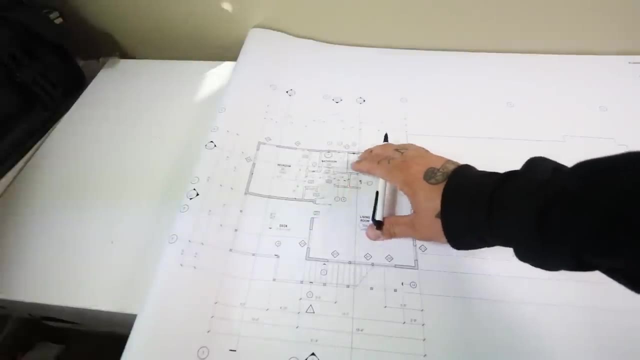 Say you need info from either the architect or the structural engineer. You're going to email or get in touch with them with what they call an RFI request for information. So say you needed info on these plans from the structural engineer or the architect. 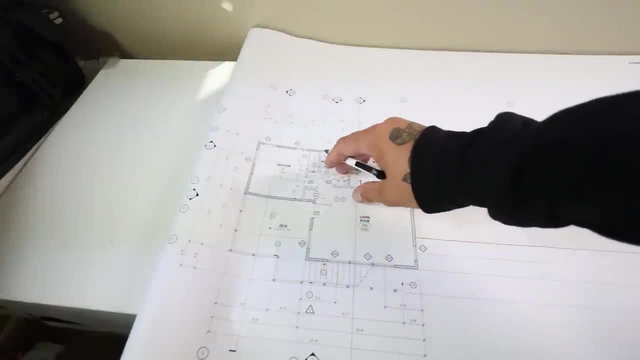 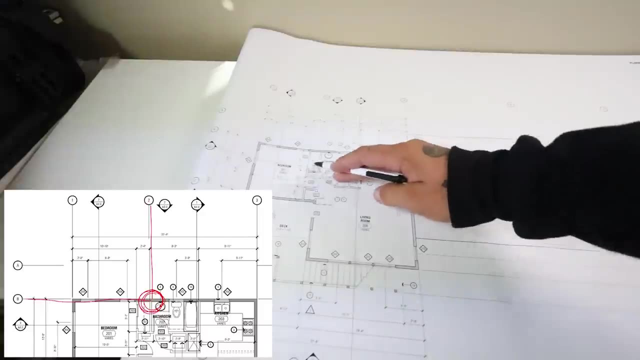 You don't want to email them and say: hey, in the bathroom by the sink closest to the wall we have an issue. You have grid line B and grid line two there. You can explain exactly where you're talking about when you send in that request for information. 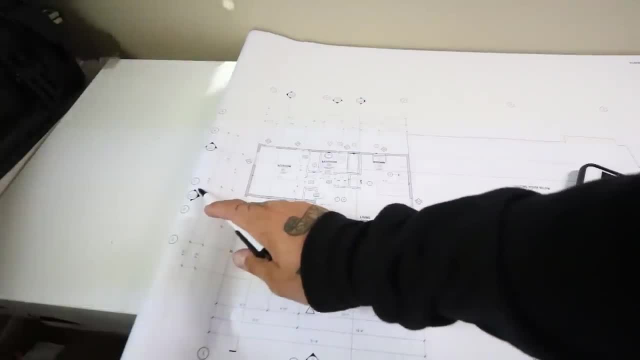 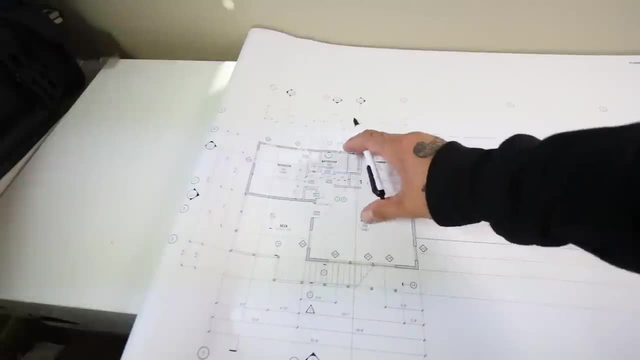 They can get back to you on a response and ask you: hey, is everything all right with the corner? See, and one right there You can verify: yeah, everything's spot on. All of this is super easy to understand And the biggest problem with people being able to read plans is not many people have. 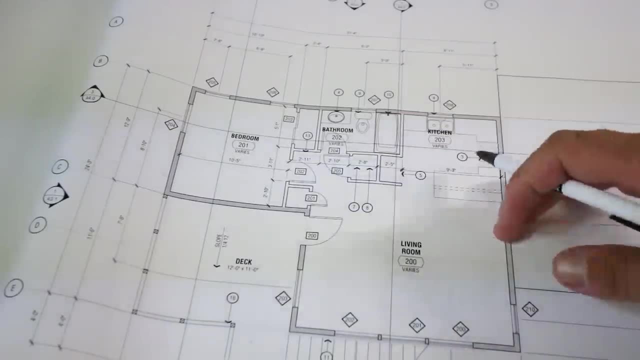 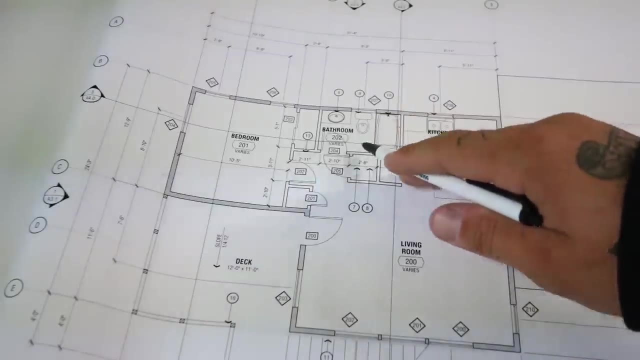 the opportunity to Same thing as below. You guys have your kitchen laid out here, Kitchen cabinetry here Looks like a little stove there, Sink goes there. Bathroom is in here, Sink, toilet tub, everything is laid out. The architect gives you info and all that. 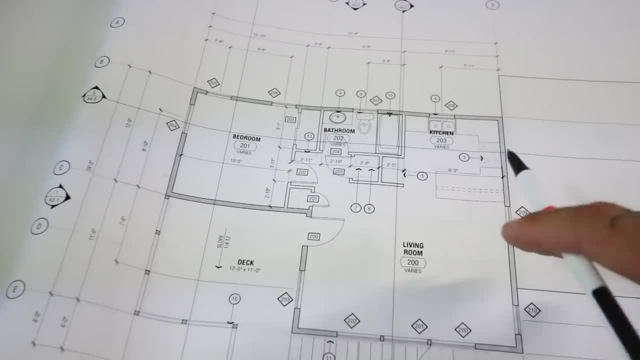 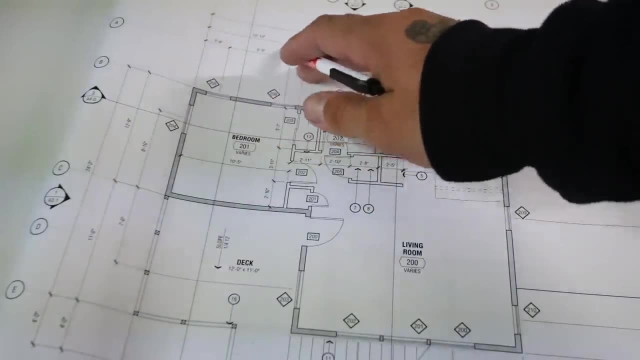 And, as you can see, the reference points for everything, For your keynotes over to the side. none of this has to do with framing. Only thing we take from this is your grid lines, all of your layout marks here for marking center of your windows and your doors. 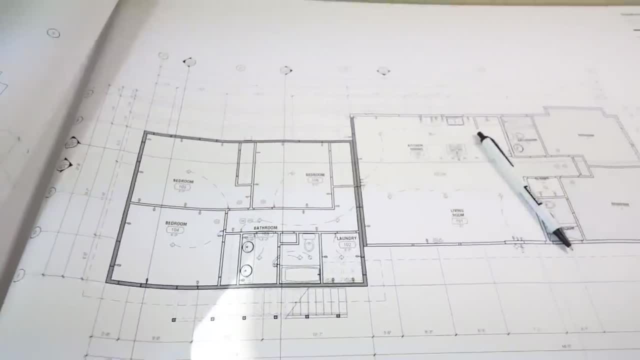 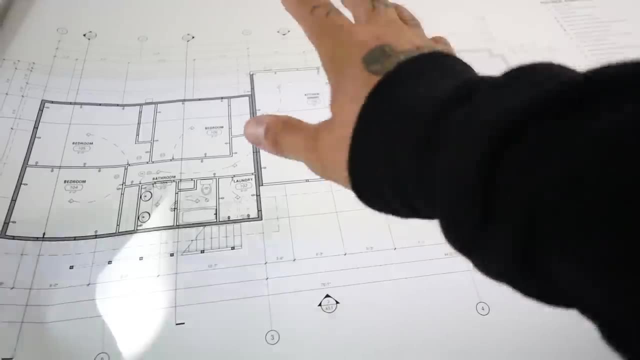 That is it when it comes to framing. Now we're going to zip through this as well. This is first floor reflected ceiling plan. This has nothing to do with us. You have an L here for your lighting, a couple of dollar signs, another crap for electricians. 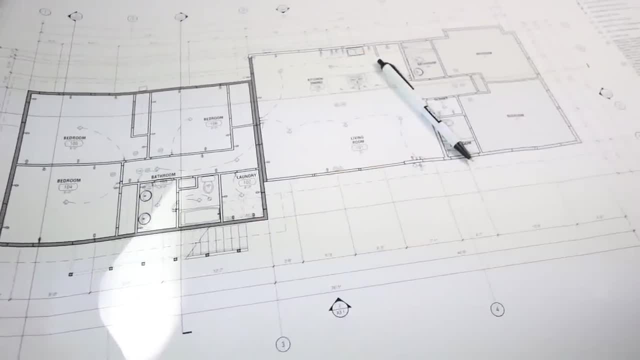 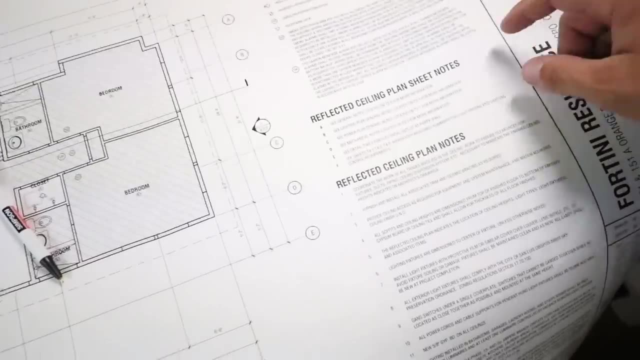 We don't need to know anything About that whatsoever. Therefore, we're going to keep on trucking, Just to where you guys can see it. in case you're curious, We have electrical symbols here. Ceiling plan sheet notes, mechanical notes, lighting notes. 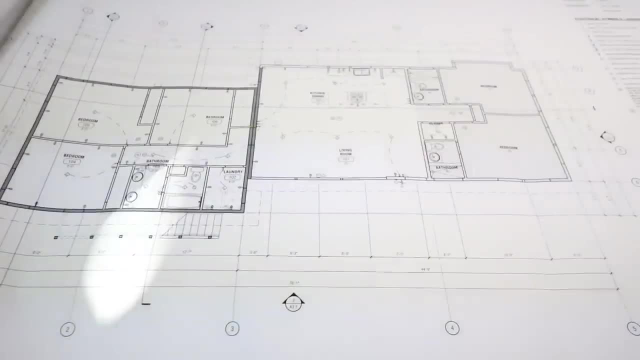 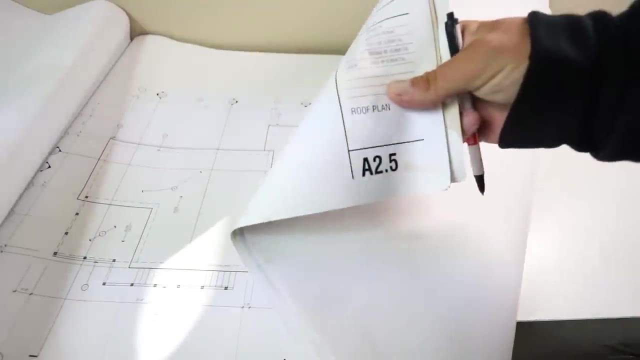 We don't do that. No disrespect to you guys, though. Have much love for all other trades. This is the roof plan here: Architectural 2.5.. This doesn't give us too much info either. It says here that our slope 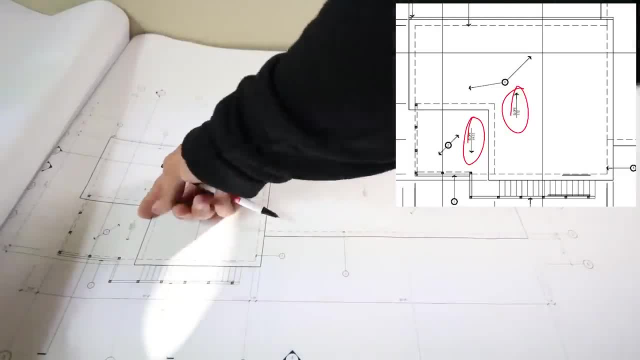 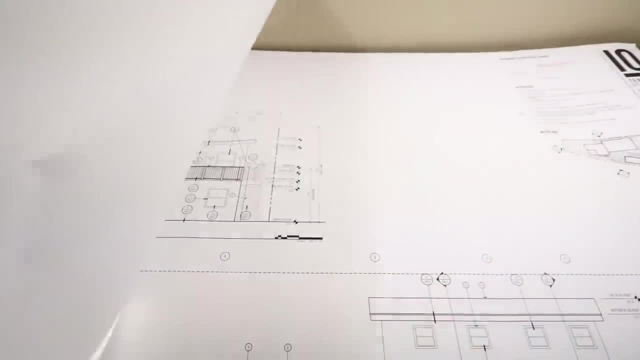 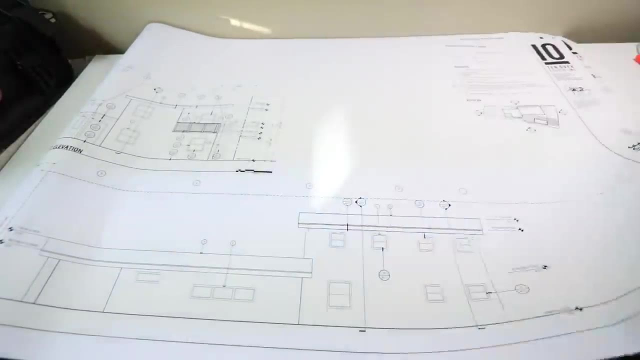 Is 1 and 12 going that direction, downward Quarter inch to 12 for our deck going that way. We already knew that info, though Not much for us here. Holy moly, We're onto something that actually makes sense. Exterior elevations: A3.0. 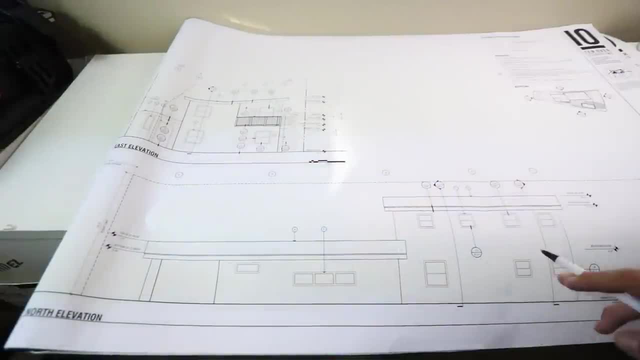 As you can see, here we have east elevations- You can see it from one side- North elevation- you can see it this way, And we've got these as well. This is where we're going to stay and talk for a second. Now you've got a scale down here as well. 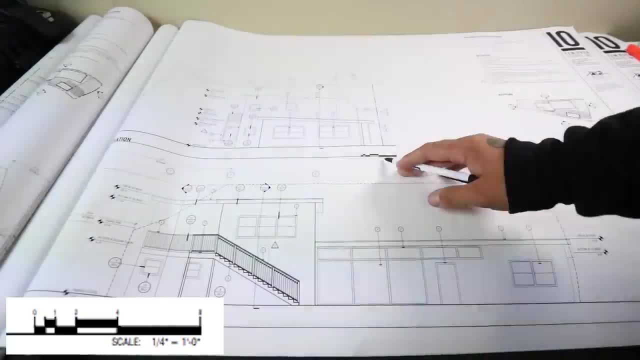 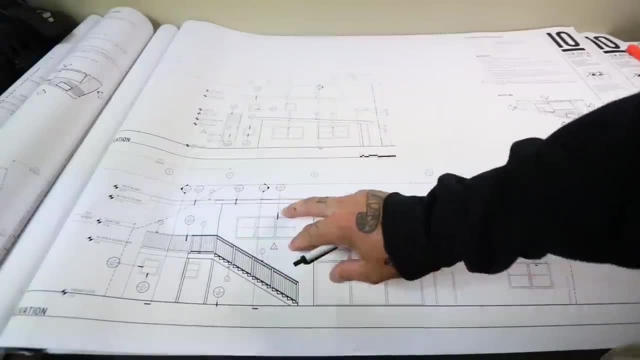 Quarter per foot. Every single page on a set of plans Will have a scale. Here we're quarter per foot. Some places will be 3, 16ths, Some 3 8ths, Depends on who draws it up. So now there are a couple reasons. 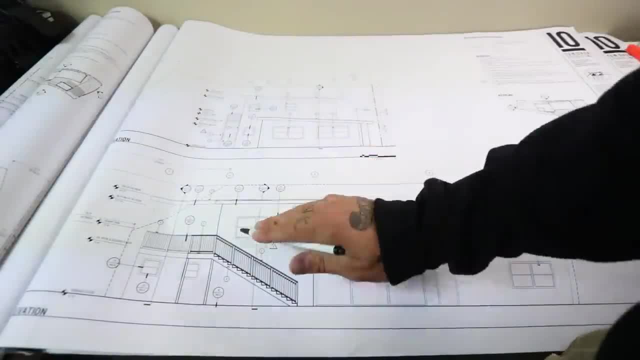 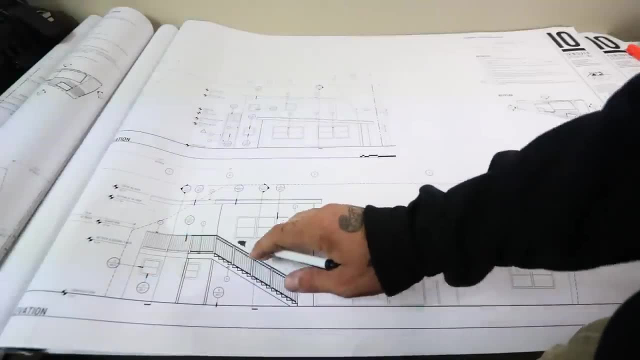 We get elevations printed out. One, it's really nice to see what you're building. And two, you have info like this: New deck and second floor at nine foot. We can only assume that we've got an eight foot wall, One foot floor system. 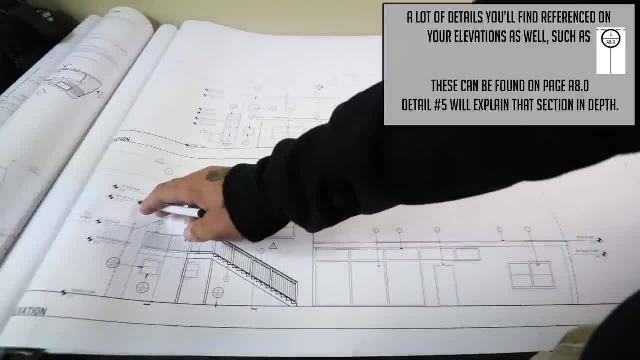 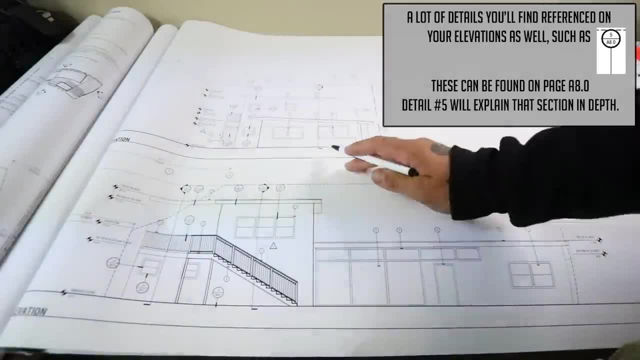 And then we go up from there, Obviously bottom of new roof 17 foot. We're going to have some custom cut studs in there, As we do have rake walls going from here Over to there. Hoping I have some time to slow down. 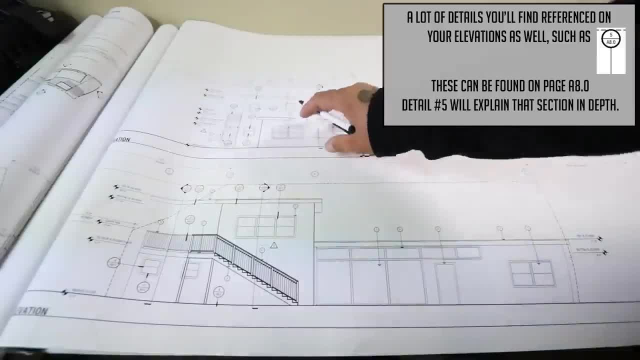 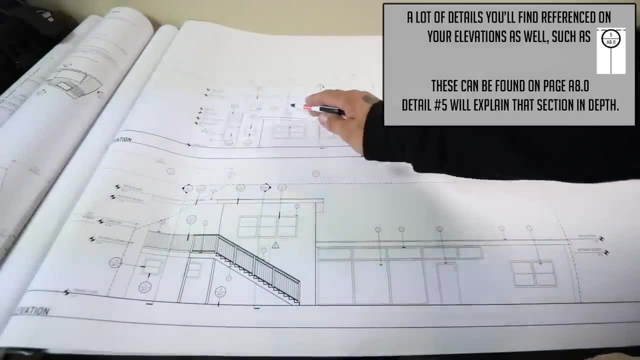 And show you guys just how to build rake walls. We can look here and assume that this is all board and batten, But we can double check that as well later on. This will give you top of new roof is 20 foot 2.. 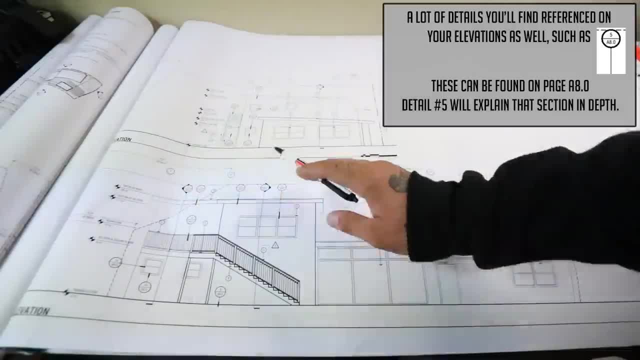 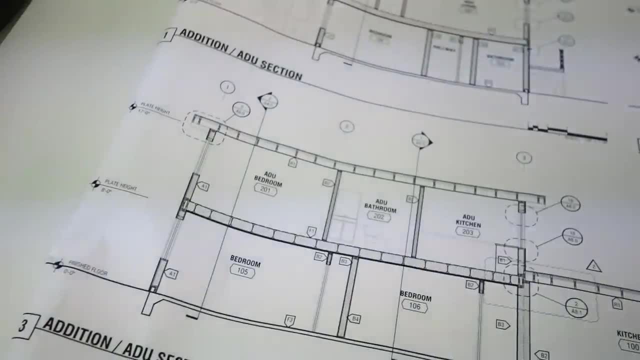 Bottom of new roof is 17 foot 10.. Top of existing roof is 11 foot. All sorts of info as far as how this place is supposed to come together. Now we're on building sections A 4.0.. Along with elevations, this will give you basic idea of your plate heights. 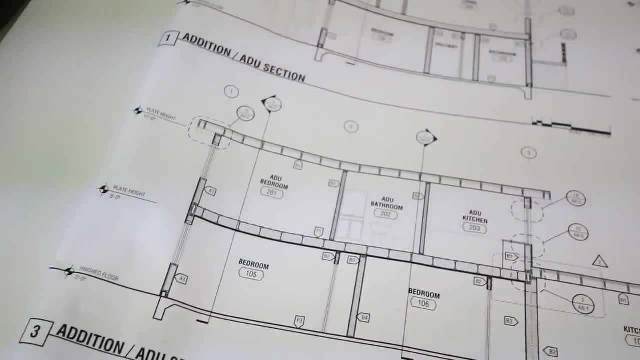 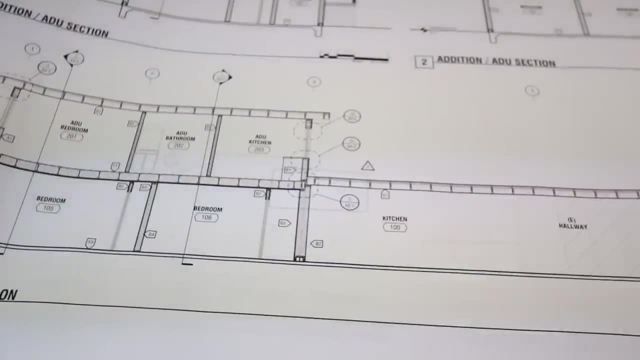 Eight foot 17 foot there. Along with that you have info on all sorts of different things Now, along with your plate heights, it gives you a basic rundown of how things are supposed to look in. here You have different reference points for A 8.0.. 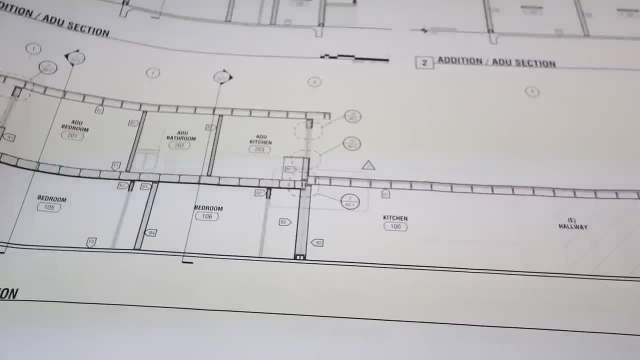 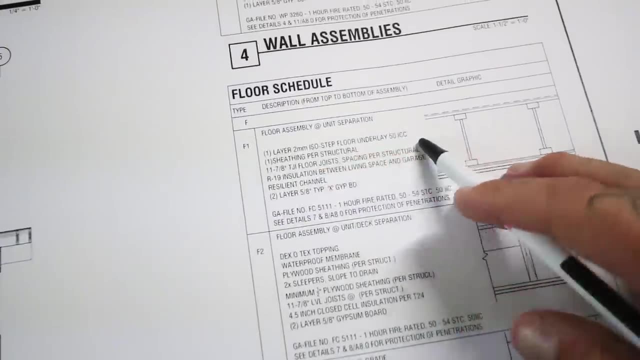 Number 10. 18. 2. You guys can flip to A 8.1 and A 8.0 and check those out. We will do that in just a second though, So on the same page it will give you info like your floor assembly. 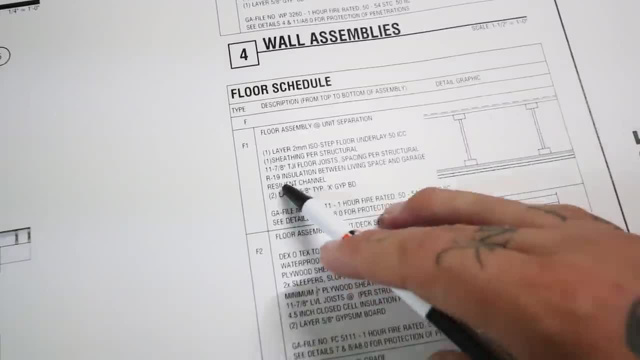 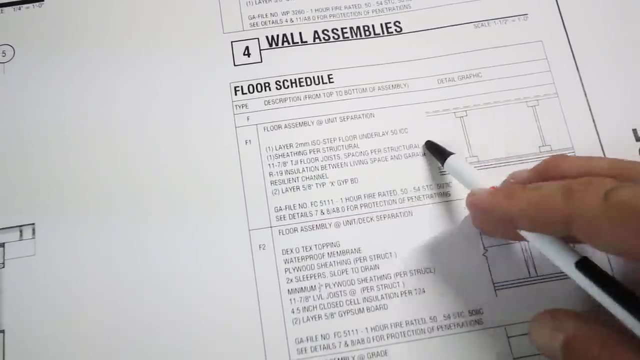 You have one layer of iso step floor underlay Right on top there. One sheeting per structural right there 11 and 7 eighths TGI floor joist spacing per structural. Gotta reference your structural to figure out how they want those spaced out. 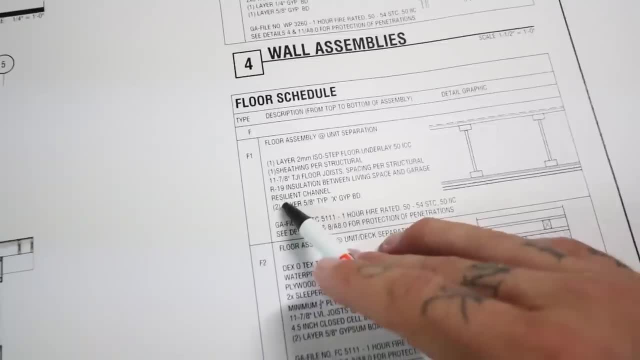 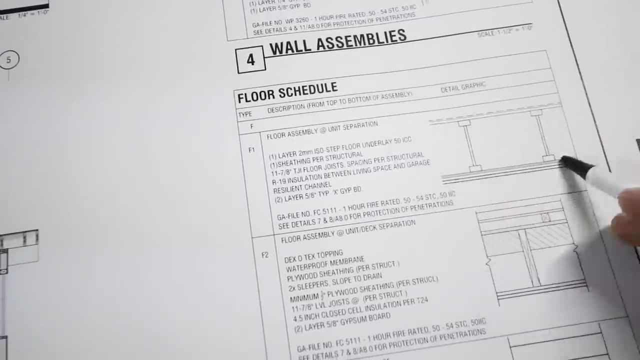 It looks like we have R19 insulation between living space and garage, A resilient channel which will be like a HAP channel, And then two layers of 5 eighths gypsum board drywall underneath For a fire block in between the garage and the living space up above. 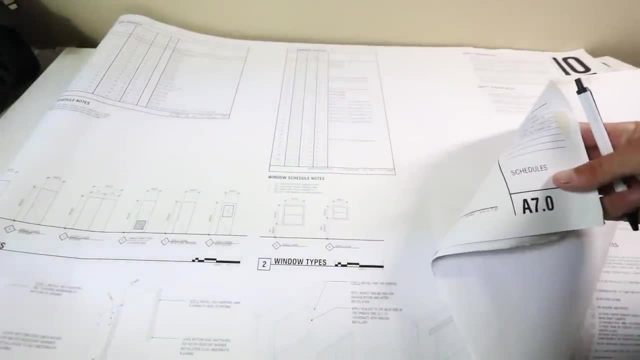 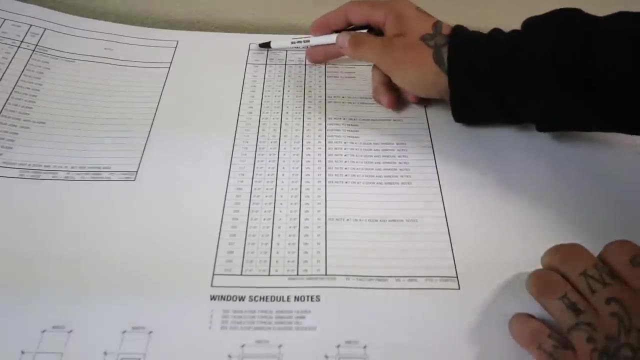 Here we go, you guys, We're almost to the end of our architectural. We are on schedules. So we have a window schedule here. You can see here, Tag all these numbers here And you have a diamond right up here. So any of these numbers that are inside of that diamond you can reference. 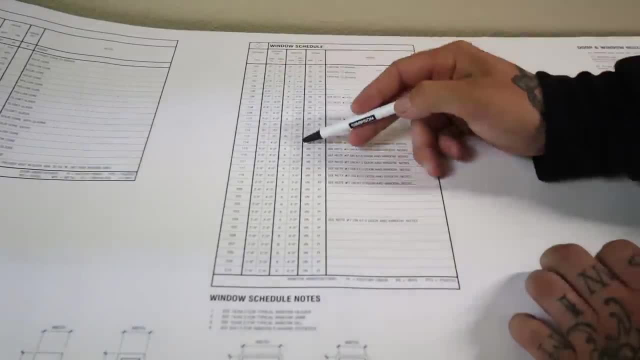 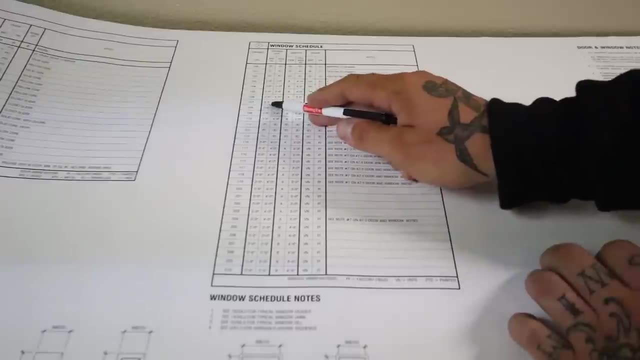 So when we do all of our plating and detailing, we have to reference this here to find out what size these windows are. Sometimes you'll have them laid out on the floor plan, Other times you don't. In this case, we have to reference here and find out. okay, this is a 3640.. 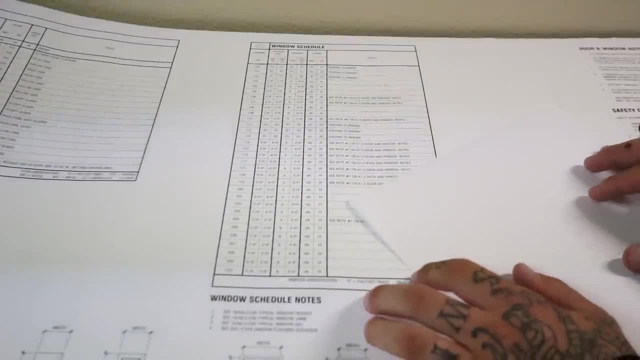 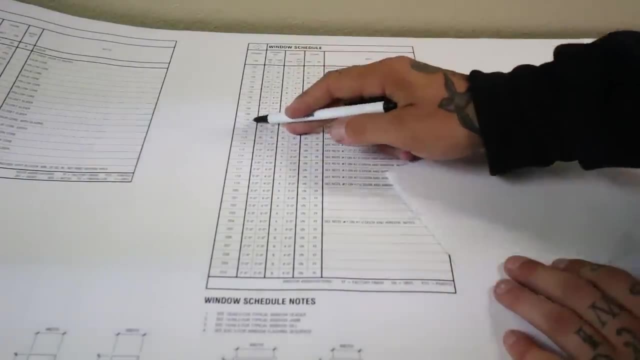 From there we can lay out So we can keep as much knowledge in these windows Videos as possible. I'm going to show you guys exactly how we lay out for our windows and our doors. Say, we have the little diamond with a 110 inside of it. 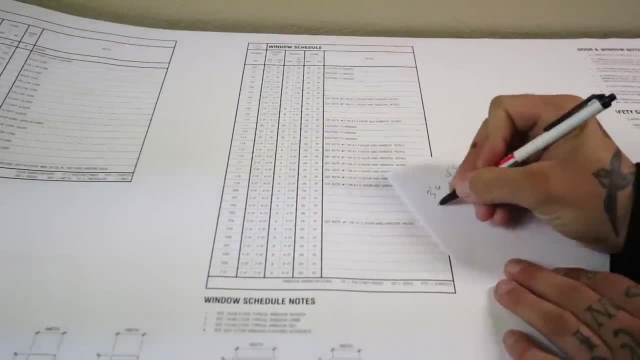 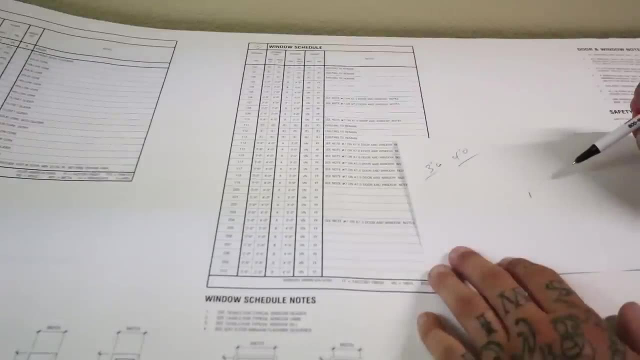 That is a 3640.. This is our width, That's our height. So when we go to layout, We'll find that center mark. based off of the numbers that we saw on our architectural floor plan, We'll find our center mark. 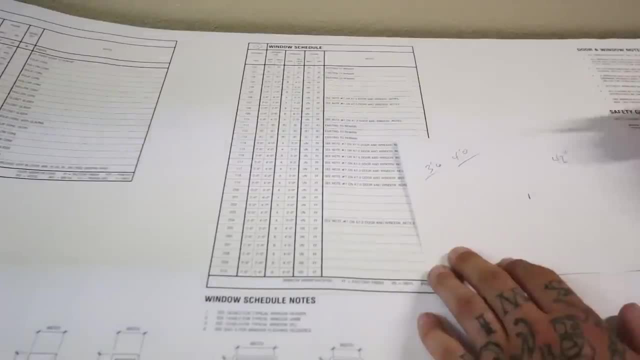 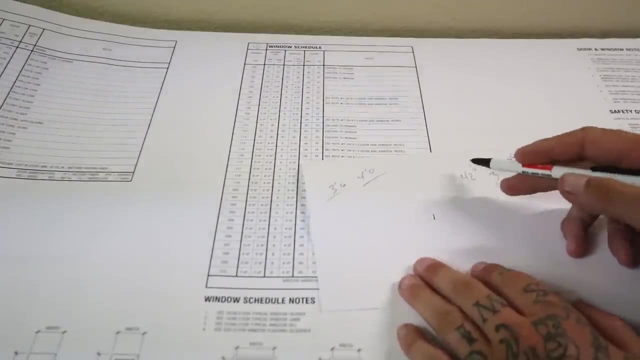 And we're going to take 3 foot 6, which is 42 inches. Now, 3 foot 6 is 42 inches. With window framing, you add 3 inches With doors. With door framing, you add 5.. In this case, since we have a window, we're going to add 3 inches to 42, making it a 45. 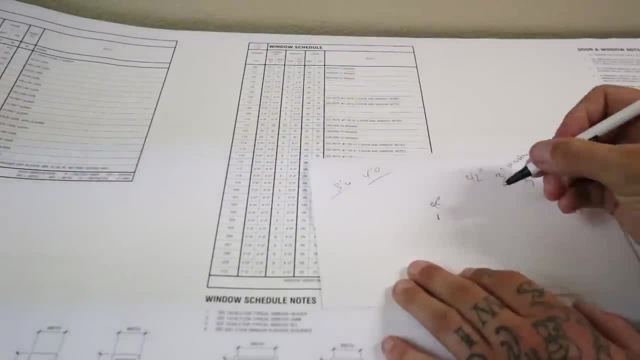 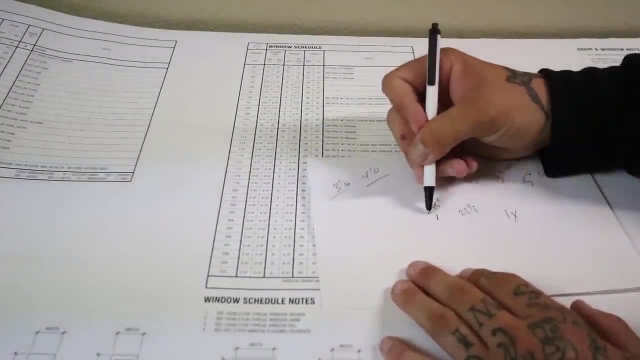 inch opening. Once you have your center mark, you're going to pull out 22 and a half inches. Give yourself a mark and a line there X, the right side. You'd pull over 22 and a half this way. Line X. So you have a king stud here, King stud there, 45 inch opening And then once your trimmers go in And if you guys label those, You will have a 42 inch opening. Let's check out our door schedule real quick. 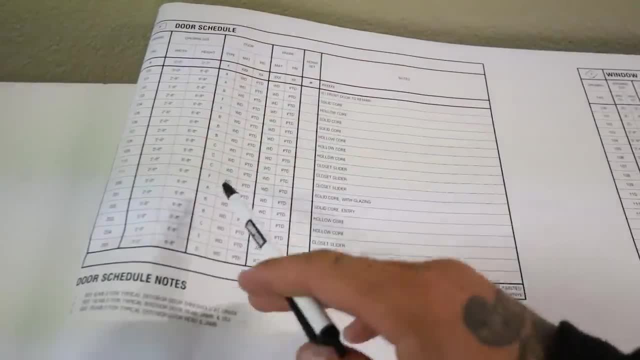 So we have similar info. You have your rectangle there. Any of those numbers you can reference here Your width: 2 6 6 8.. 2 6 6 8.. I'm going to show you, guys, how we layout our doors. 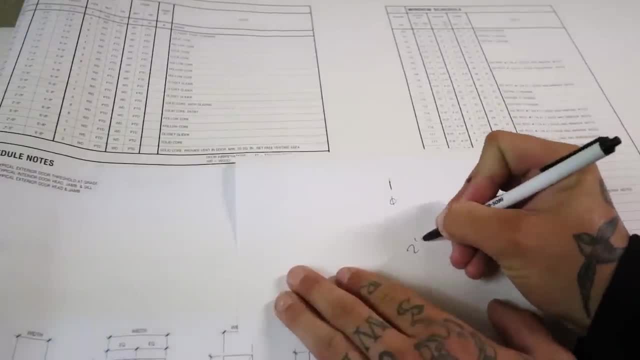 Same thing goes for doors. You're going to find your center mark And say you're working with a 2, 6, 6, 8.. 2, 6 is 30 inches. Now you add 5 inches when you do doors. 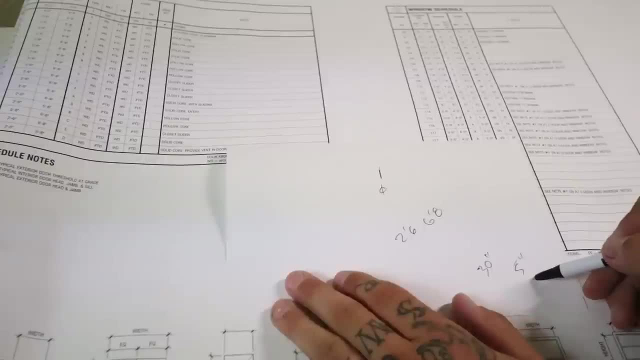 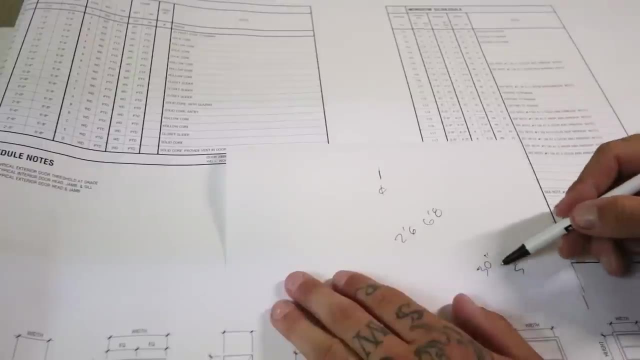 And the reason you add 5 inches instead of 3, like the windows, Is you have your 3 inches for trimmers on both sides And then you have 2 inches- 1 inch on both sides for your casing. So in this case, 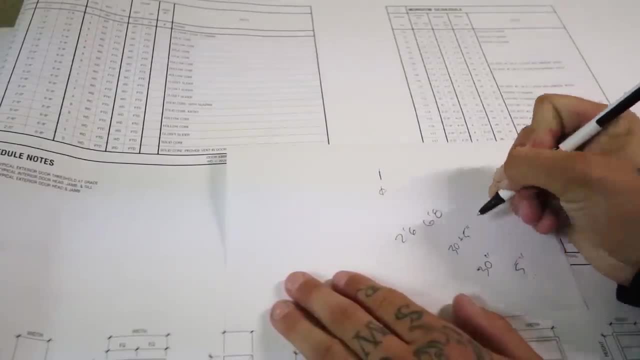 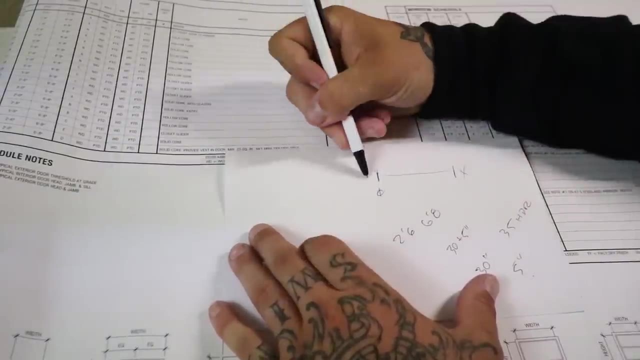 You would add 30 plus 5 inches. You'd end up with 35. And that's what your header is going to be. You'd come out 17 and a half. Give yourself a mark and an X. Come out here. 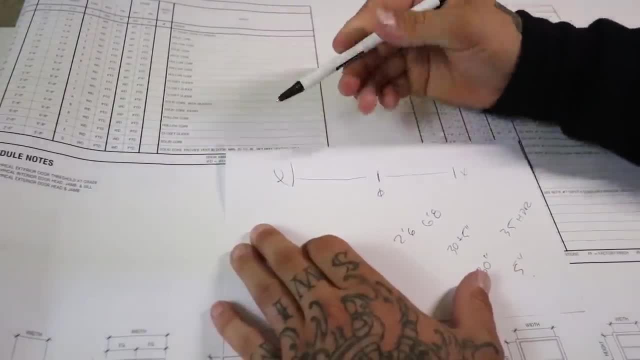 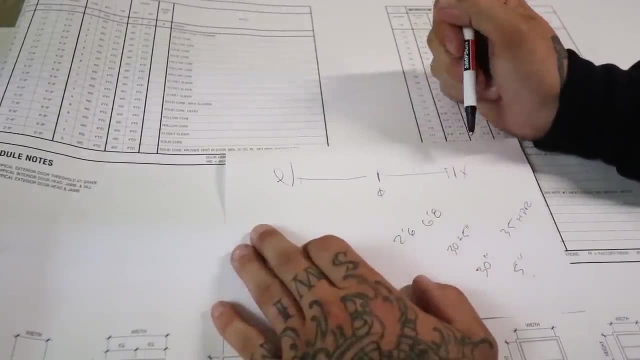 Mark X: You have a 35 inch header that goes in there Once you add your trimmer. Your trimmer, That leaves you with 32 inches- 1 inch on both sides for your casing, And then your door goes in between. 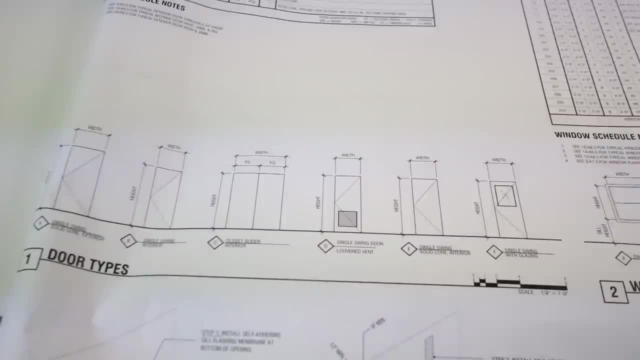 So now you guys know exactly how we layout our doors And our windows. In our door schedule we have different types of doors: A, B, C, D, All the way out until F. This is actually a really important section here. 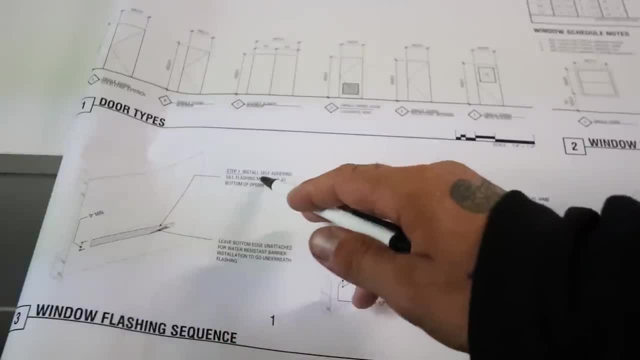 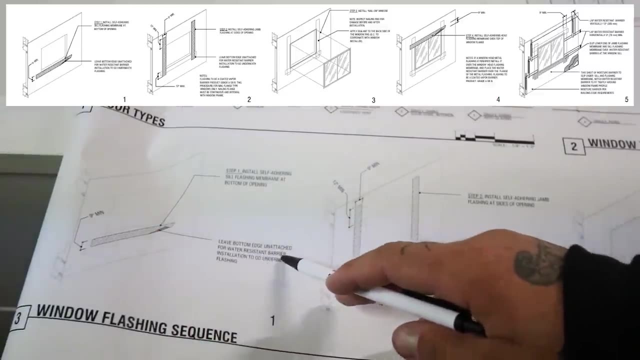 And I feel like a lot of people should watch this. You have your 9 inch Self adhering sole flashing membrane at bottom of opening. You leave the bottom unstuck, As you can see. Leave bottom edge unattached For water resistant barrier installation to go underneath. 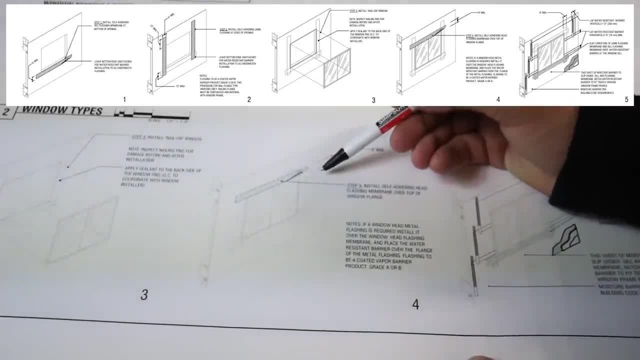 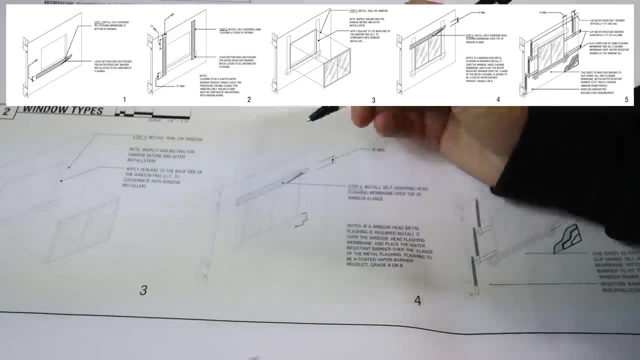 Now this is done So many different ways, But the way that they're recommending it on this set of plans, Once the window is installed, You're going to go ahead and paper, But you want to paper underneath That section there, But over to the window there. 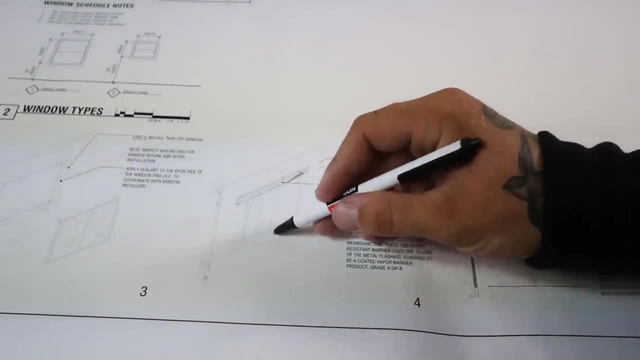 So the paper would be on top of all the flashing here But underneath the flashing there. That way, in the case that water did get underneath, It would go out on top of the paper. Now, the best piece of advice I ever got told is: 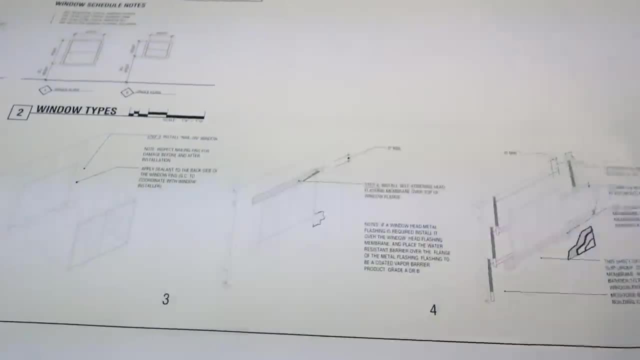 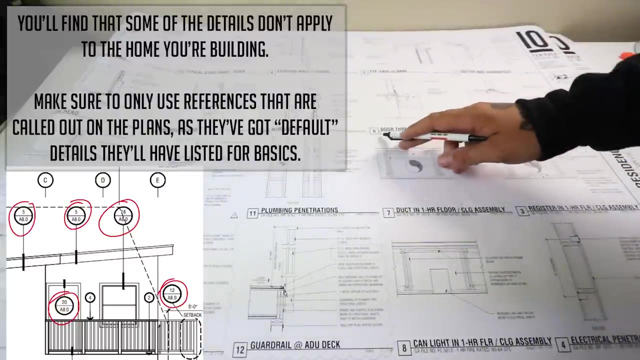 Think like water. Now we're on to One of the last pages for our architectural. We have details, Reference number 6 to A8.0.. You will have your door threshold at grade. This will explain to you guys multiple different things throughout the build. 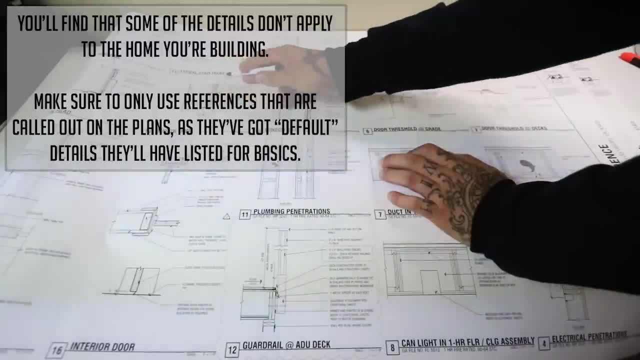 Now those reference points are awesome. to look at Number 13 here: Typical stair tread and riser, It'll give you info: 10 inch minimum tread depth, 7 and 3 quarter inch max riser. Now things like number 9 here: 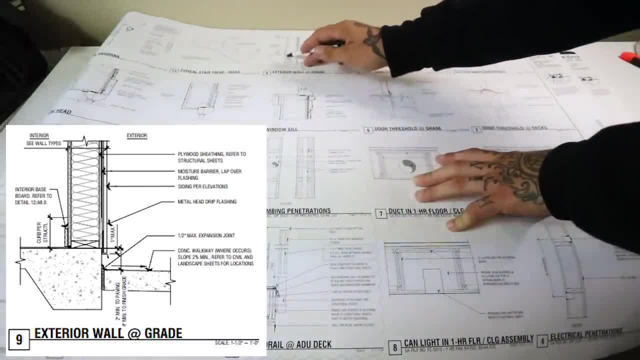 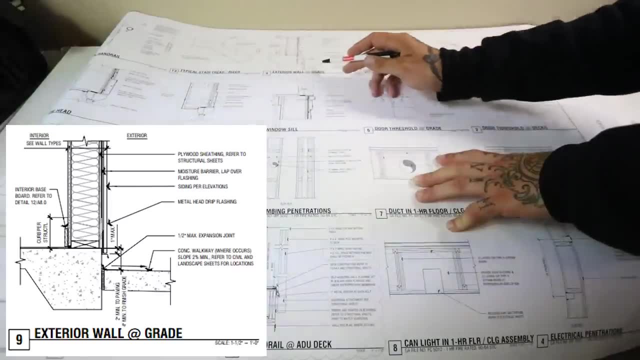 Exterior wall at grade Will give you guys an idea of where things are supposed to be. As you can see, We have our 2x6 wall here. We have our plywood sheathing- Refer to structural sheets- Here on top of the concrete. 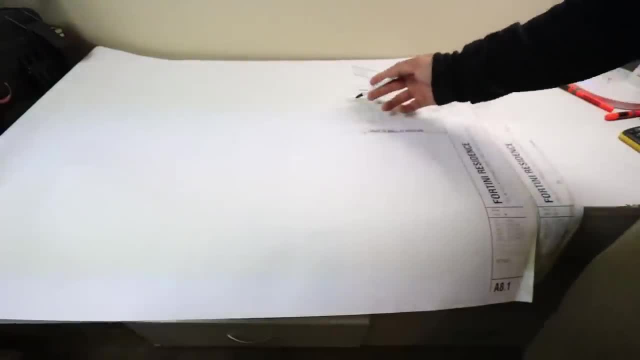 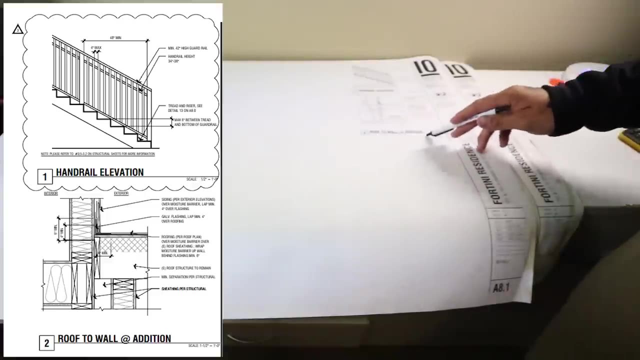 And our siding goes on the outside there. This is our last architectural detail And that just didn't fit on the page before, So they included it here. This tells you things about the handrail elevation And the roof to wall at addition. 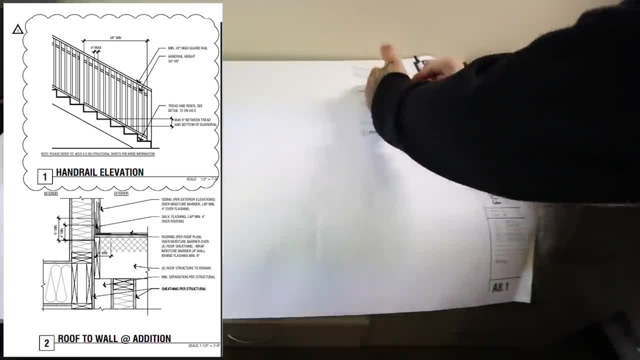 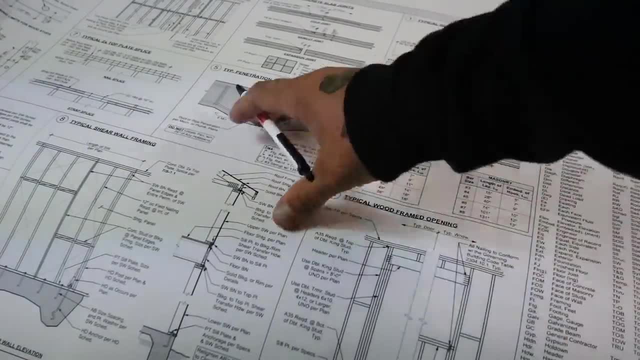 This will tell us our connection from existing into our new stuff, All stuff we should be looking at, But in my opinion, though, The architectural is the easy stuff, The structural. here is where the fun begins. So we are completely through with our architectural. 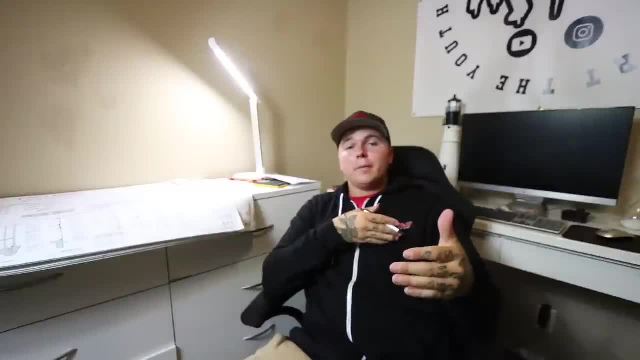 You guys have a pretty good understanding Of how to not only snap your lines on your slab But lay out all of your plates, Detail all of your plates. I showed you guys how we lay out our windows, How we lay out our doors. 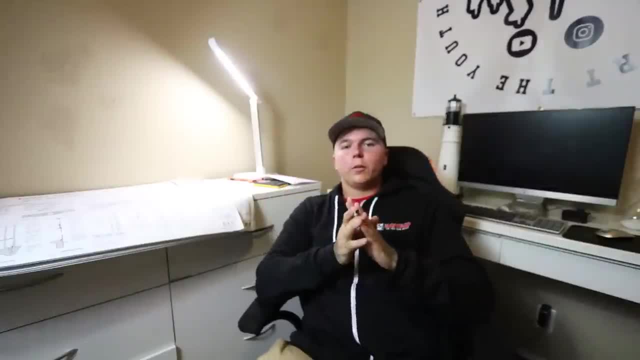 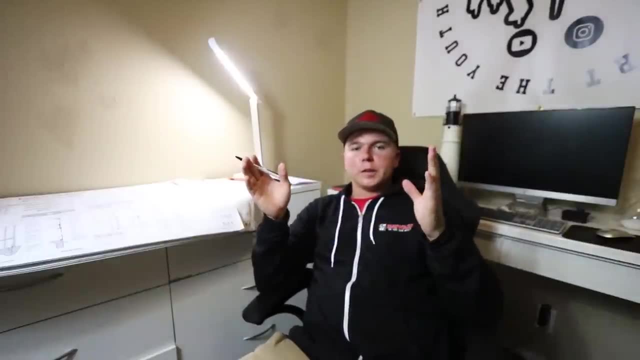 And you guys remember, there's always a golden rule: Ask the person you're building for, though, We do 3 inches for our windows, 5 inches for our doors. As I explained, the 3 inches is just for trimmer on both sides. 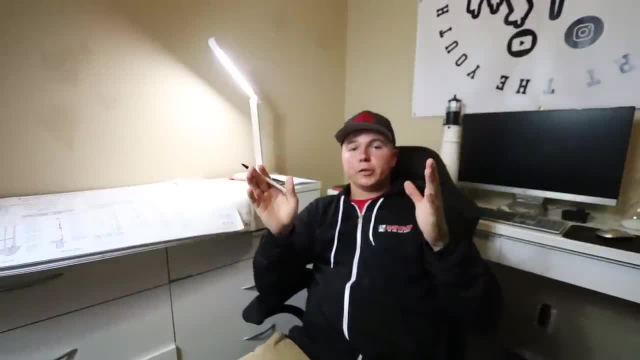 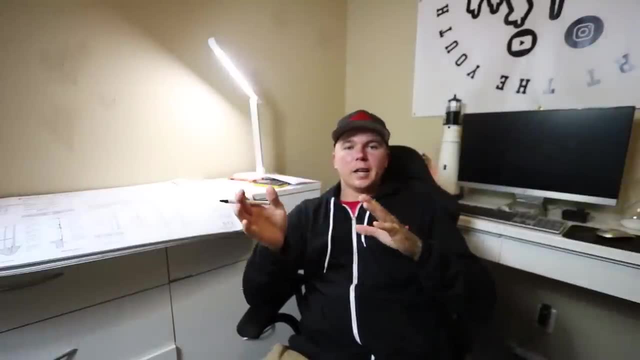 And the 5 inches on the doors is for trimmer on both sides, 1 inch casing on both sides. I showed you guys the A8.0 and A8.1.. Which are nothing but details From the side view, The front view. 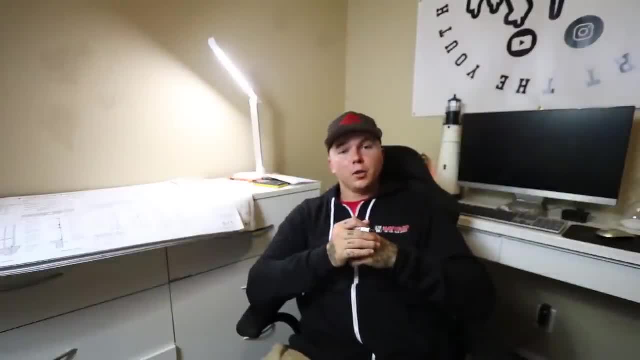 Showing you exactly how it's supposed to go together. As we saw, we have 2x6 fascia Smooth out. We have a block with 4, 2 inch diameter holes. Insect screen along the back. We know that that's going to be a vented block. 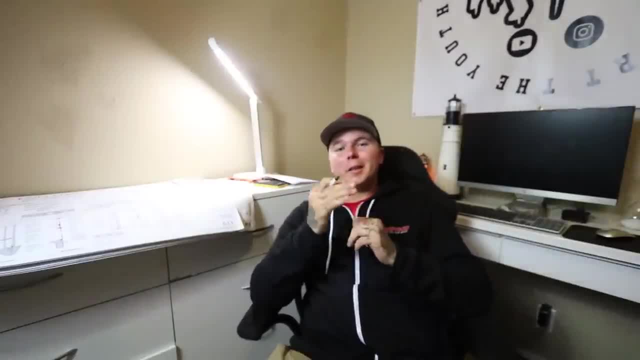 And the biggest problem that I've found Is a lot of people don't know how to read plans Because they've never had the opportunity. My best advice to you, If you've never had the opportunity To sit down and look through a set of plans,